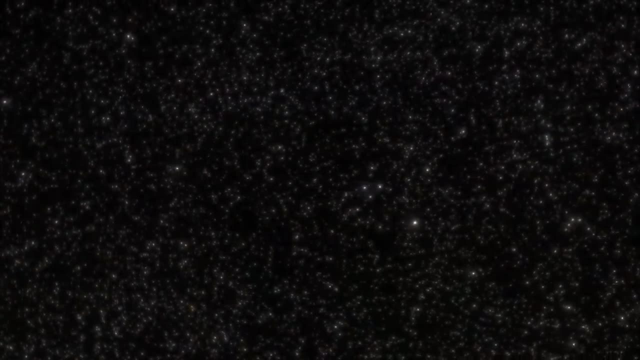 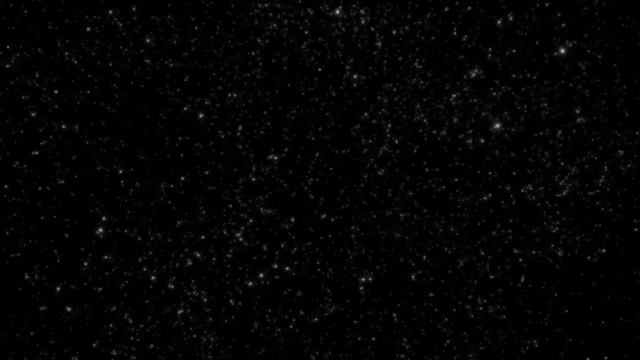 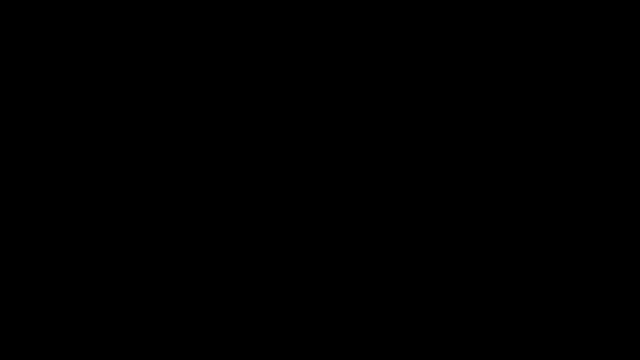 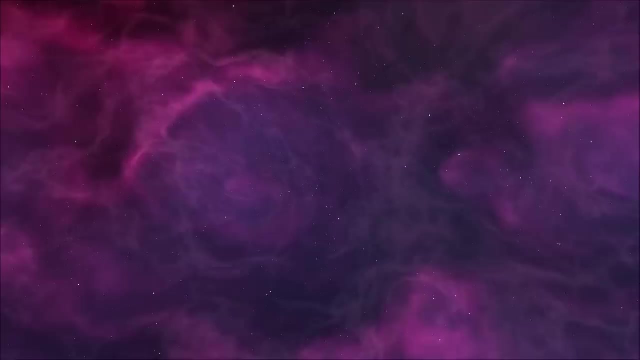 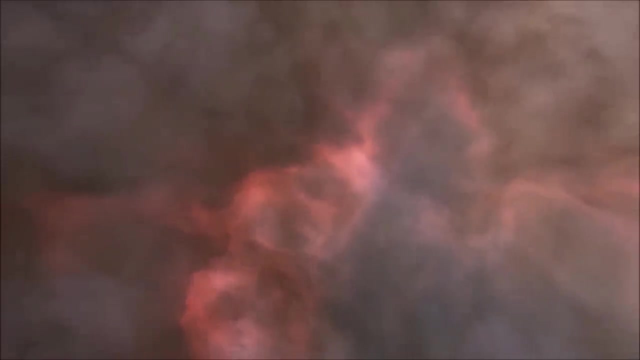 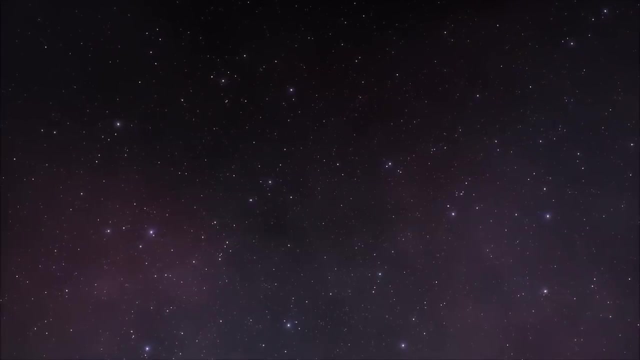 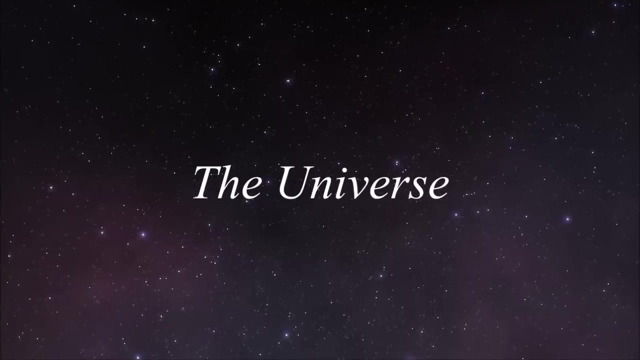 of the universe's unprecedented scale, which could be hundreds, thousands or even millions of times more voluminous. This is our universe's story. The first thing to consider is language. What do we mean when we say the universe? The universe is defined as all of space and time. All points in space are all points in. 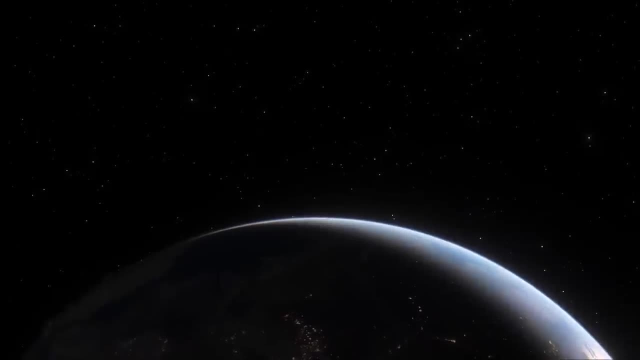 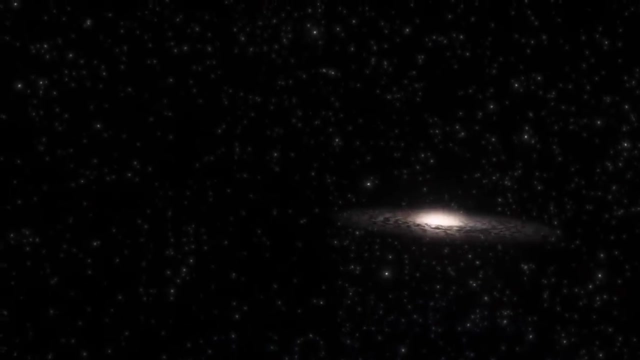 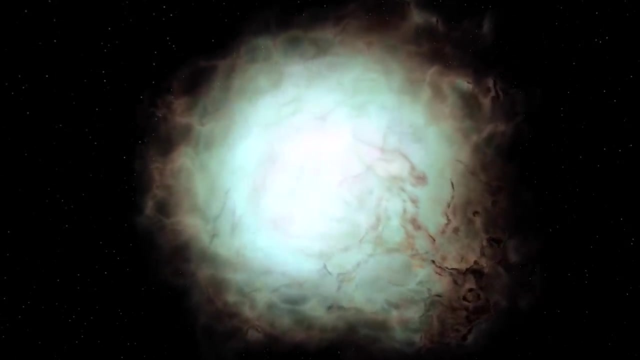 its life. Space is the volume within the universe, the three-dimensional field which lies beyond Earth's atmosphere, acting as the vast backdrop to the universe's matter. Time is the constant flow of cause to effect within this space, the catalyst of life, death, creation and 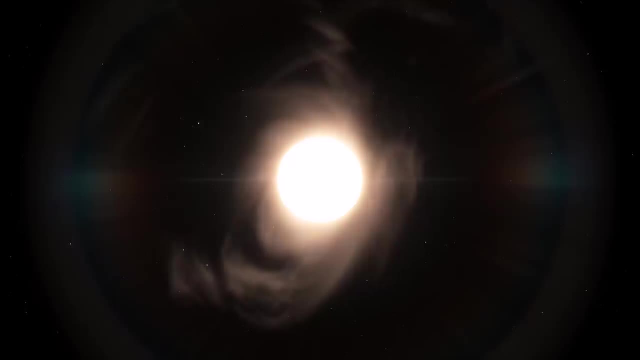 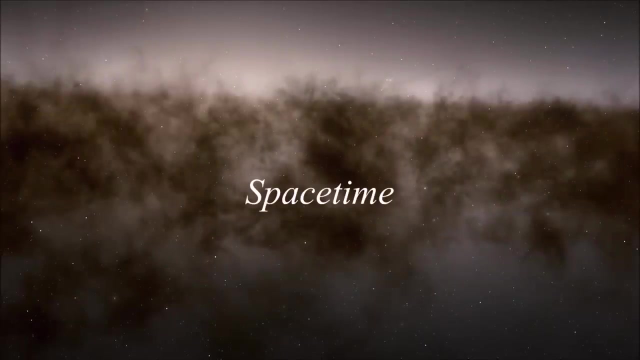 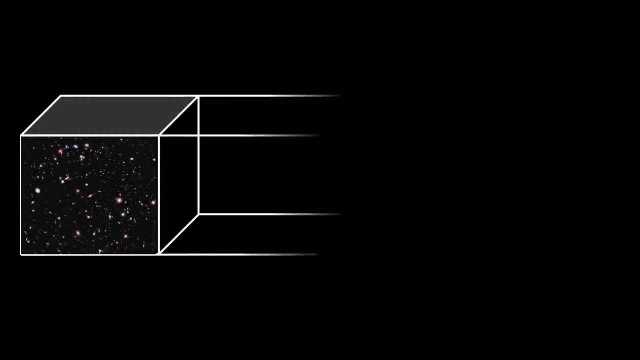 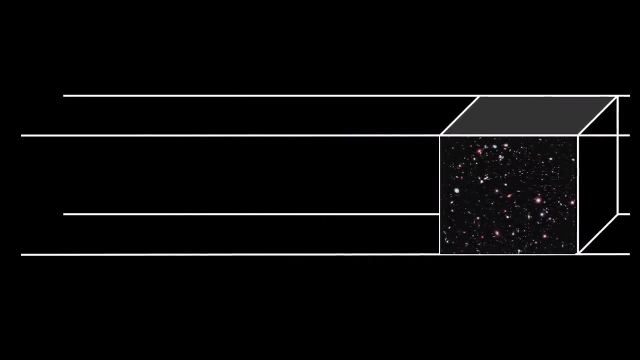 evolution, Space and time are fundamentally linked and they combine to form a system of nearly unknowable complexity known as space-time. In this model, space constitutes three dimensions and time is the fourth dimension, and any 3D cube cross-section along this axis represents the universe at a certain point in its life. 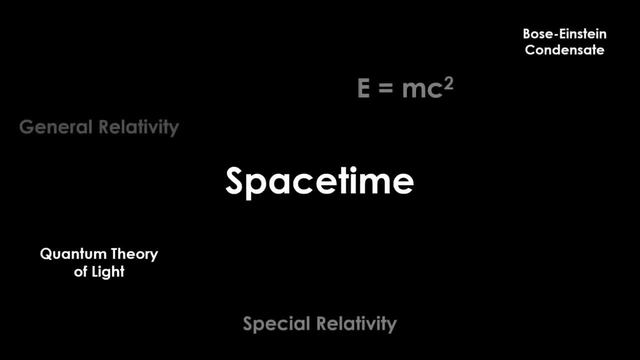 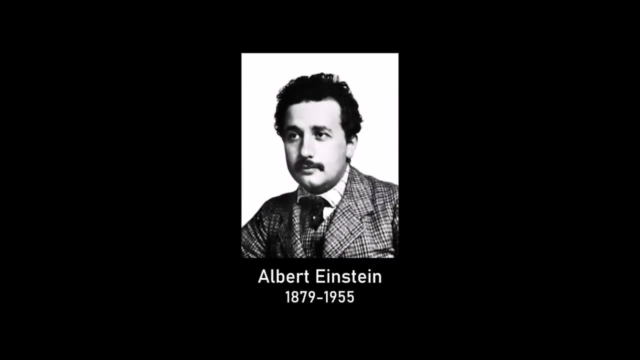 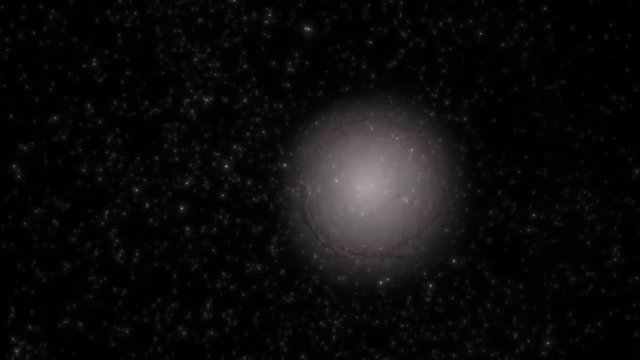 Our understanding of space-time, and a great many other scientific ideas, can be traced back to this man, Albert Einstein. He understood space and time in a way that nobody had done prior, giving us two fundamental frameworks with which we model our reality today. 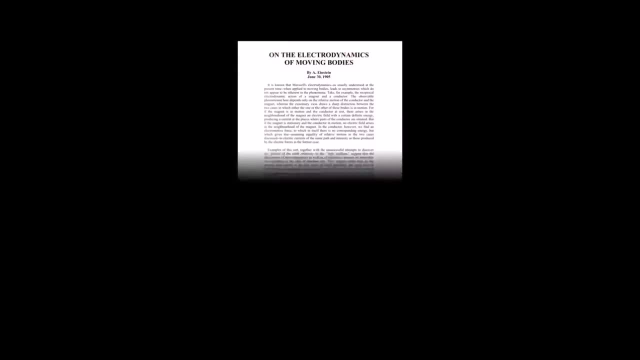 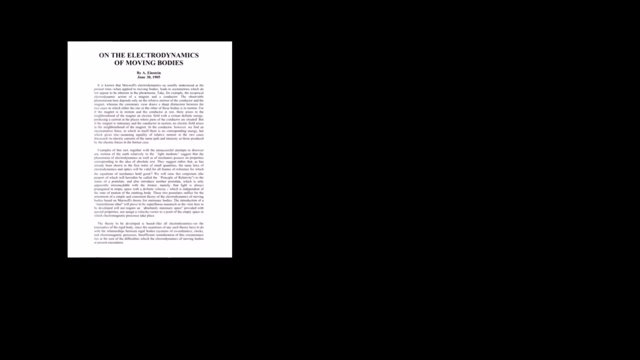 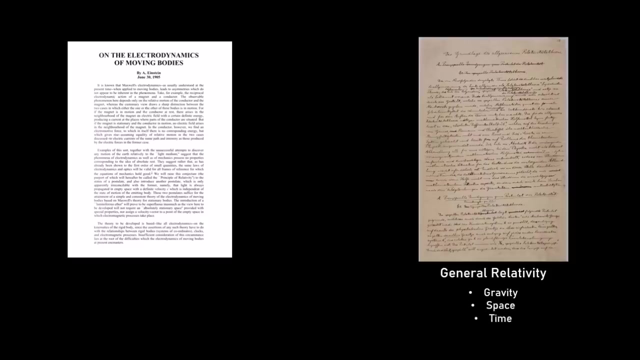 In 1905, Einstein presented his theory of special relativity, changing the way we view light, mass and energy. Then, in 1915, he presented his theory of general relativity, a comprehensive interpretation of gravity, space, time and their links. These elegant 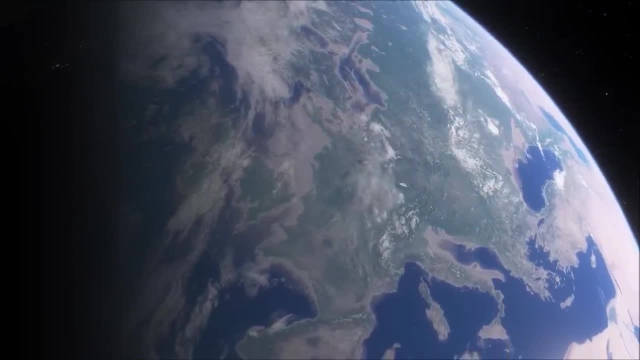 theories have survived in science for many years and have been used for many, many years and have been used for many, many years. These elegant theories have survived in science for more than a century and they underpin a lot of what we know about the universe today. 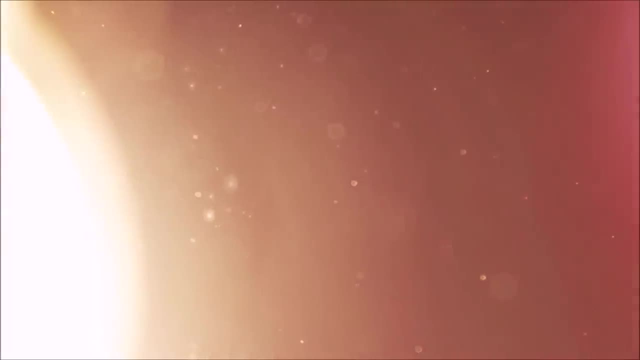 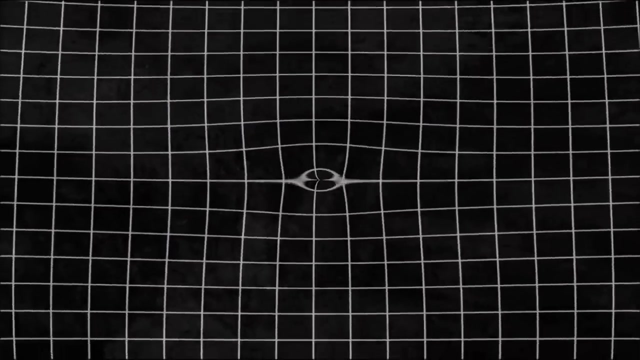 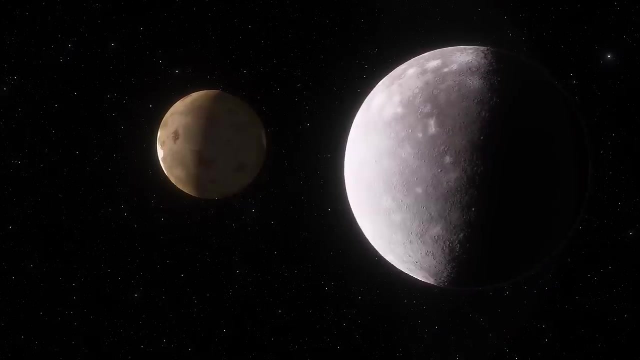 According to Einstein, mass is a form of condensed energy which has a warping effect on the flat plane of space and time that lines our universe. The resulting curvature on this flat plane is felt as gravity. Gravity is the effect of objects of mass attracting one. 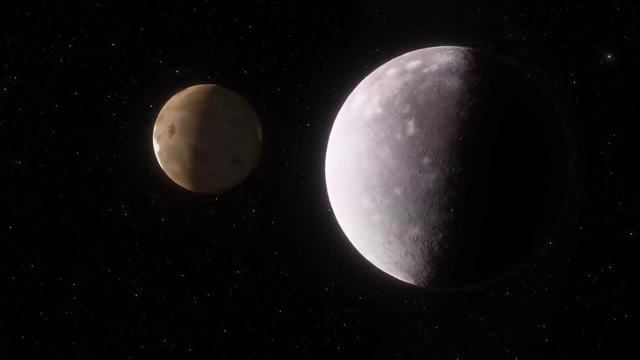 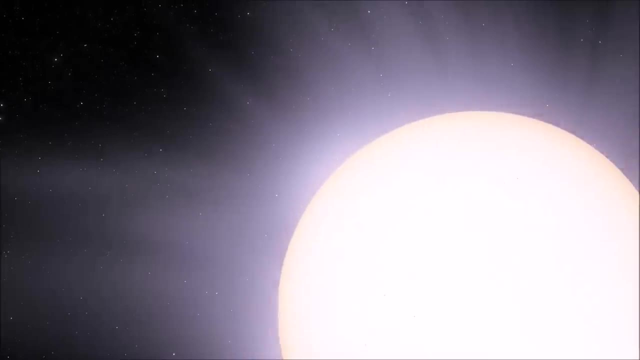 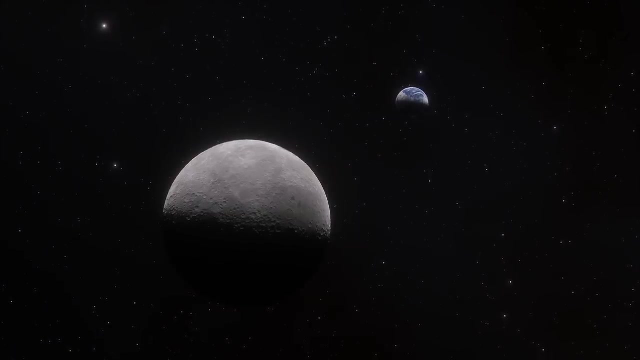 another by distorting space-time. It is the simplest yet most profound way of determining the fundamental forces which govern our universe. We don't need anything special like heat. All we need is mass. If you have mass, you have gravity And as such, it dominates the 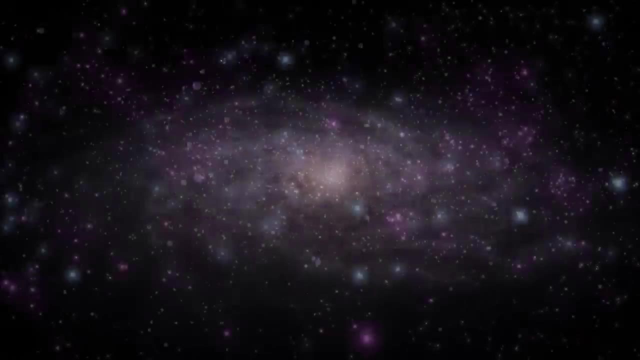 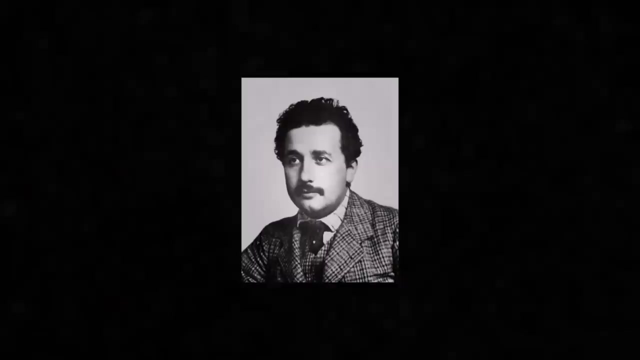 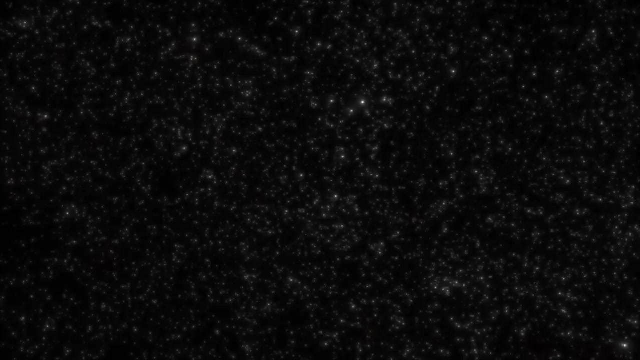 behaviour of the universe at all levels, from the small particle-level interactions to the large-scale behaviour of galaxies. Our understanding of the latter owes to this man, Edwin Hubble, an American astronomer who was not afraid to take on the biggest questions, making a number of ground-breaking. 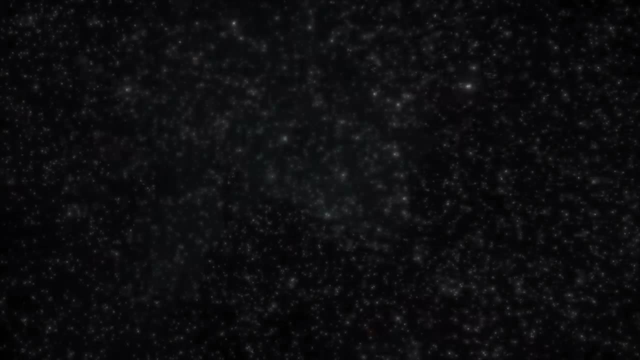 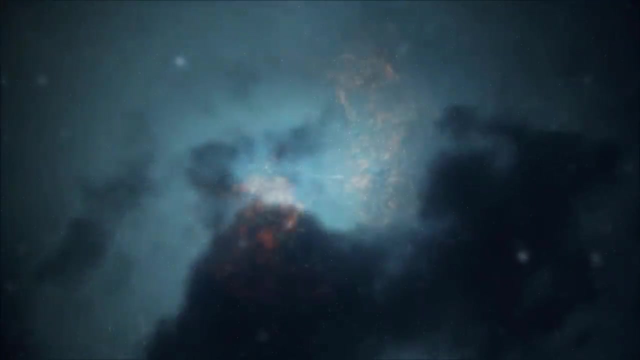 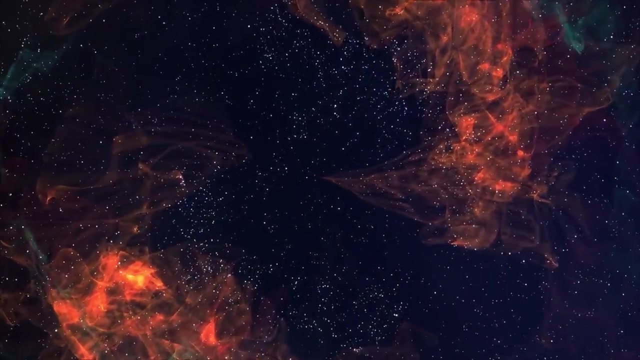 discoveries Before Hubble, it was believed that the universe was static, in that it was neither expanding nor contracting and was populated entirely by stars and nebulae in every direction. However, in late 1924, Hubble found that one such so-called nebula was actually 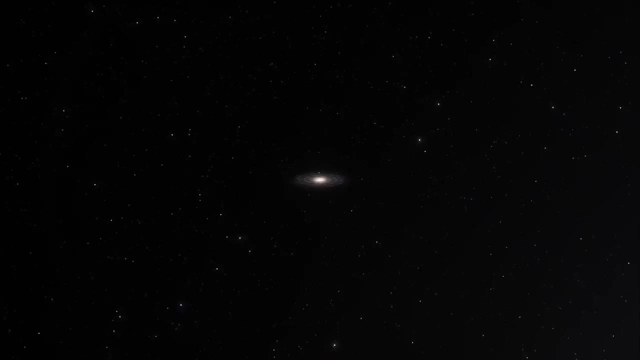 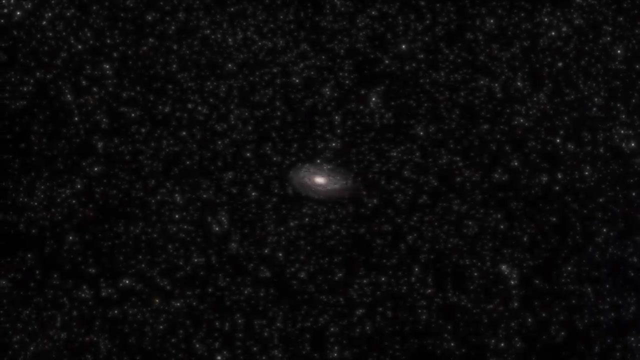 a separate collection of stars, like the Milky Way, but much further away from the Milky Way. The Milky Way is a galaxy, but much further beyond than originally thought, leading to the revelation that the Milky Way galaxy is in fact part of a larger universe of thousands. 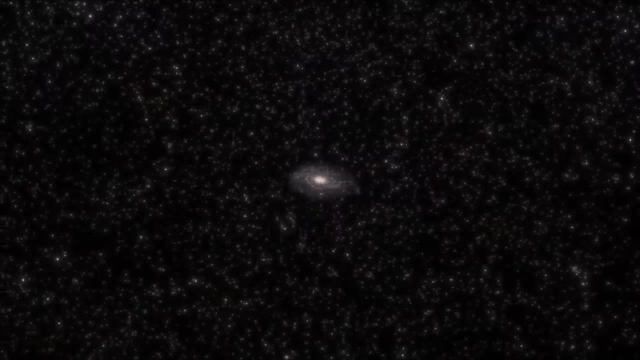 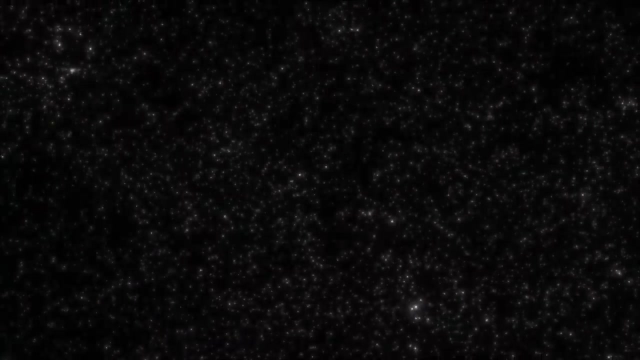 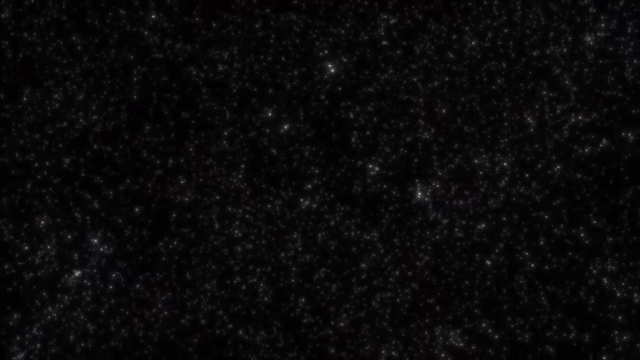 or perhaps even millions of other galaxies By the end of the decade. in 1929, Hubble then followed this up with one of the greatest discoveries of all time- that the universe itself is expanding and not static. These revelations, along with Einstein's theories, 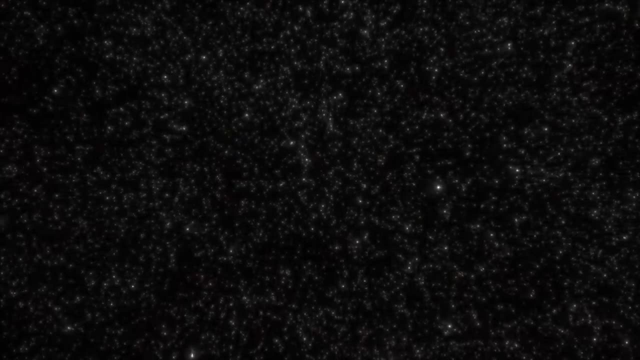 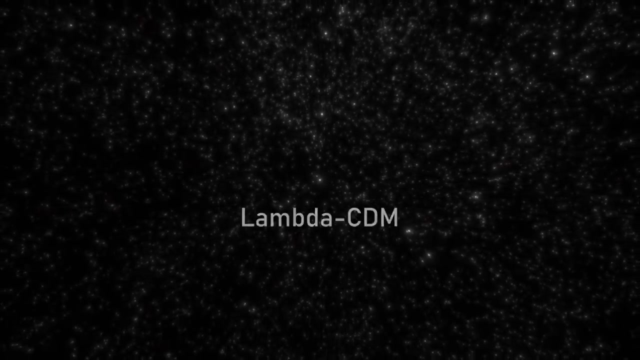 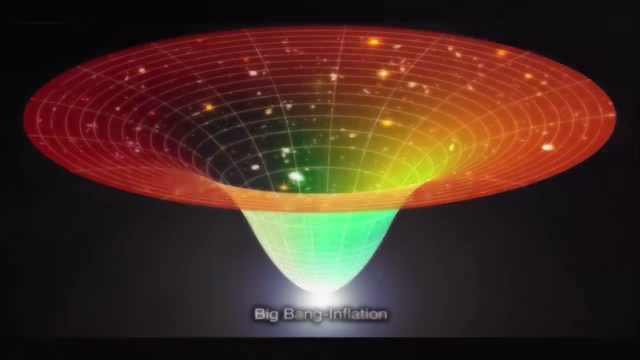 and the work of some other great scientists have all fed into our current model of cosmology- the Lambda Cold Dark Matter Model, or Lambda CDM. This is a well-established and documented model for cosmology, admittedly not without its shortcomings and unanswered questions, but it is still our best effort at comprehending. 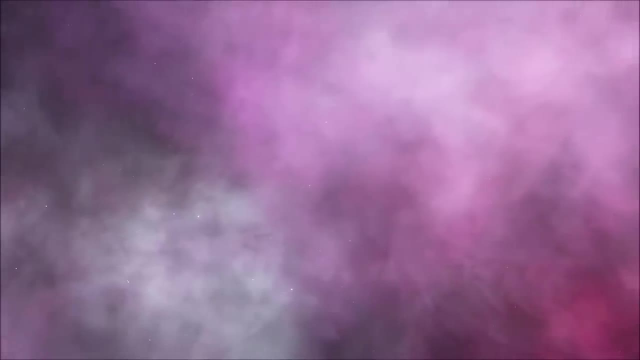 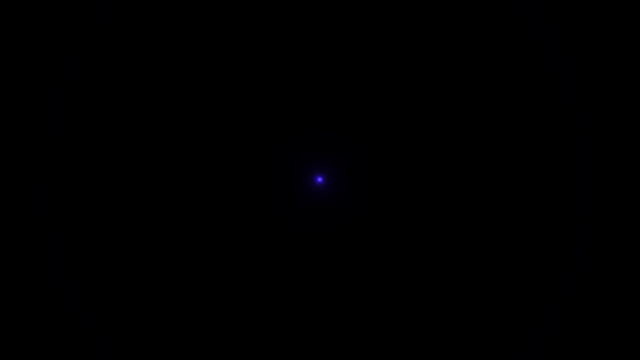 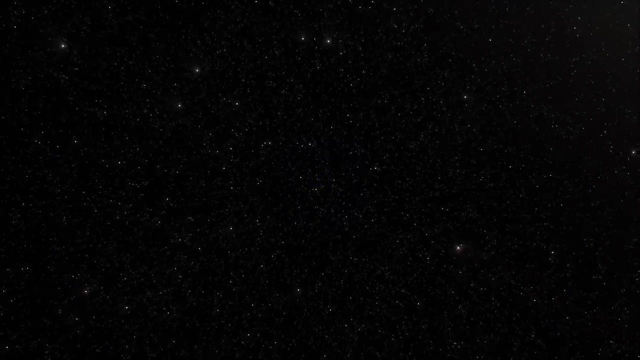 the origins and nature of the universe. nonetheless- so far, that is Central to it all is the Big Bang Theory, the idea that the universe began as a point of extremely high density and pressure, Because we know that our universe is constantly expanding, if you trace this ongoing process. 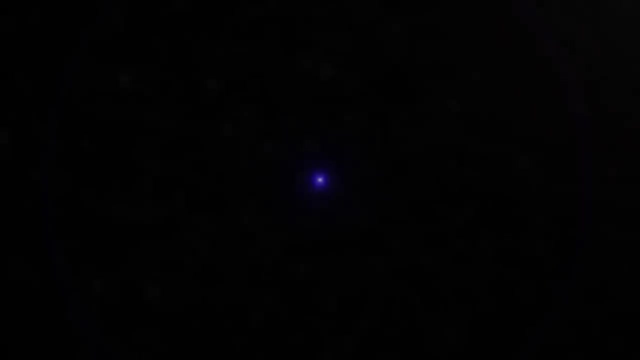 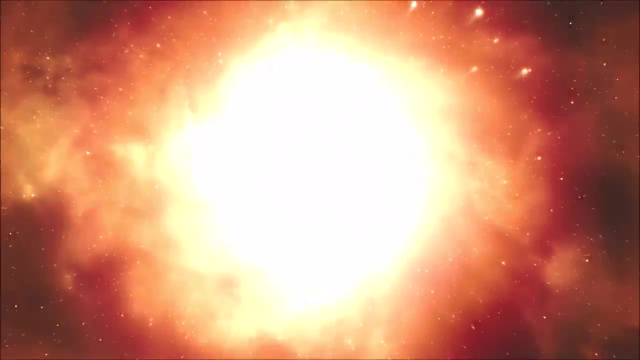 back to the beginning of the universe. you come to a point where the universe was microscopic and compressed, before it suddenly began to expand. We're not sure how or why, but there is good evidence that, at the very least, the universe was much smaller and hotter around. 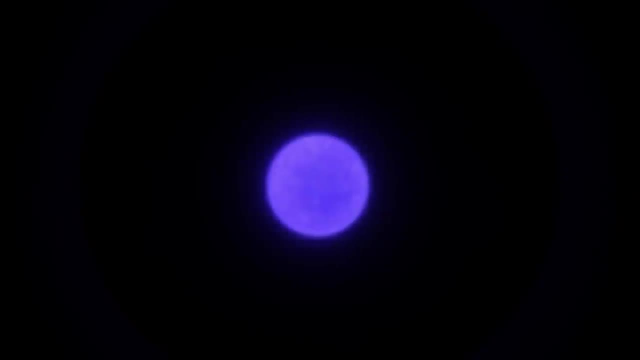 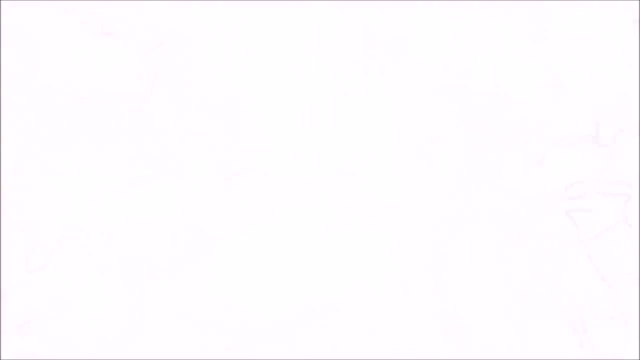 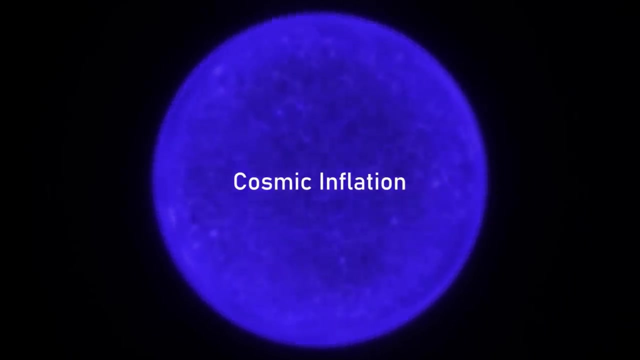 13.8 billion years ago. The time preceding crosses into the untestable realms of physics, but we believe that in the earliest nanoseconds of the universe's life, something caused it to suddenly and radically expand in an event known as cosmic inflation, bypassing the benchmarks of all. 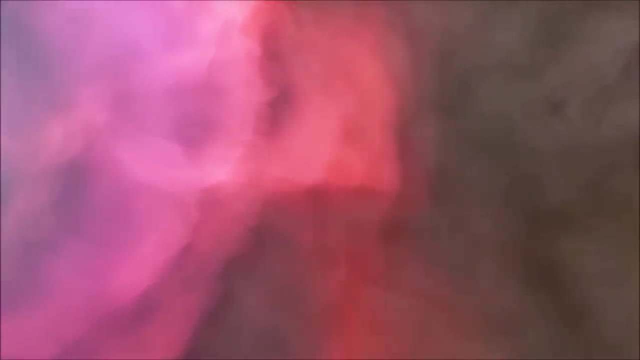 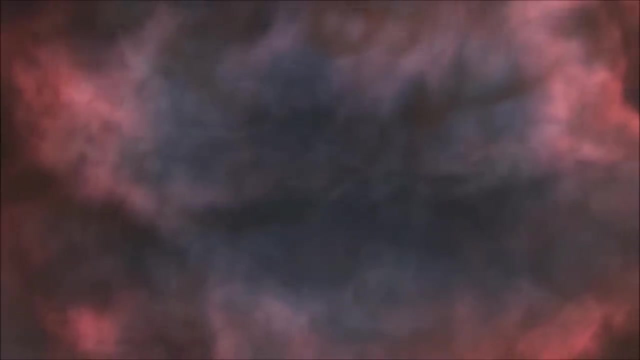 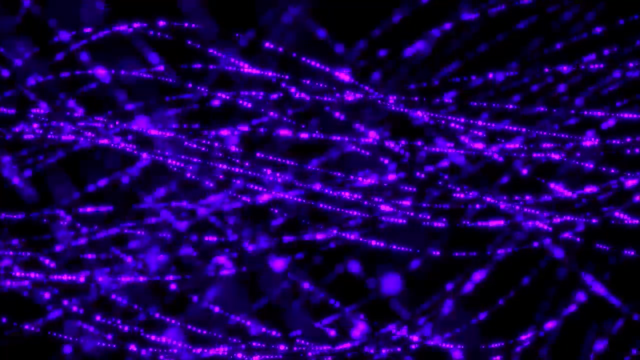 known, speeds and laws changing the universe not in size but in scale. The tiny universe as it was in that moment was enlarged, scaled up by a factor of the power of at least 10 to the power of 78. in volume, Every nanometer of space was stretched. 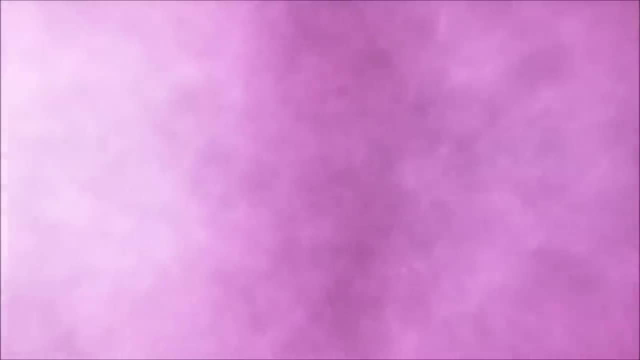 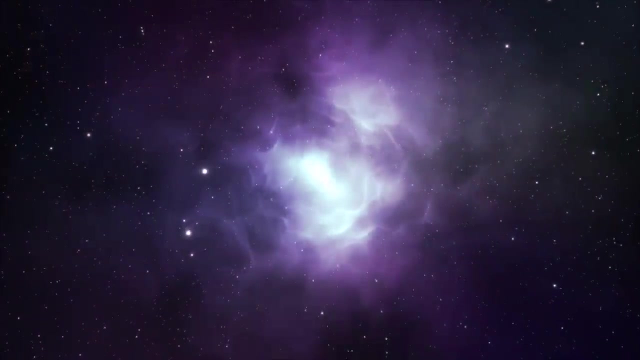 to over 10 light years, and all of this happened in under a fraction of a second. We're not sure what the total expanse of the universe was after this inflationary epoch, but what it meant was that the universe's interior was suddenly spread apart much more. 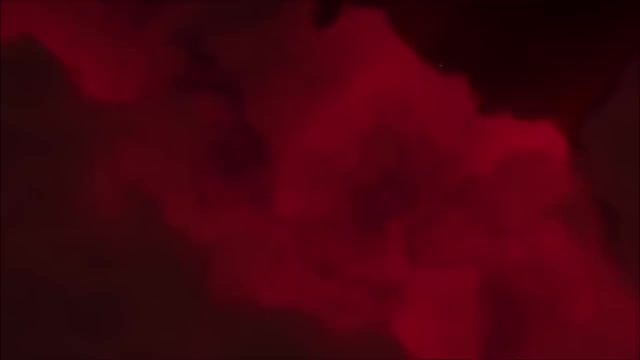 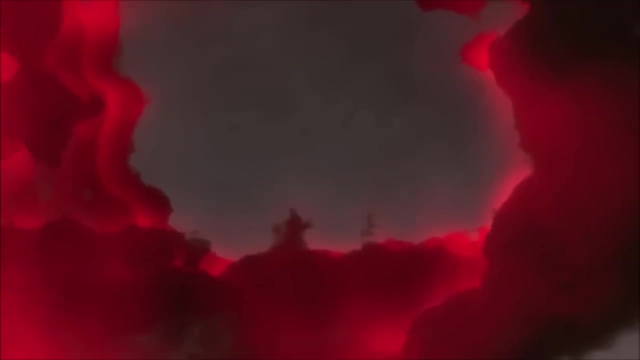 sparsely, giving its primordial energy a lot more room for things to happen. After inflation, the universe was gradually expanding. The universe was expanding, but it was expanding, and as the temperature of the universe continued to fall, the energy within condensed into. 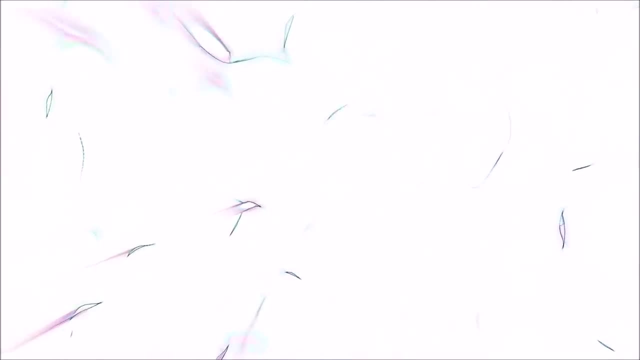 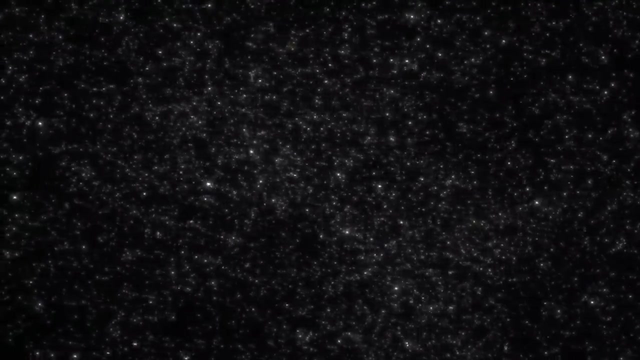 a giant universal plasma and from there decayed into the first particles and then into subatomic particles like protons and neutrons. Fast forward almost 14 billion years and the universe is now huge and brimming with much larger and richer structures. Atoms have collected into clouds of gas and gas clouds. 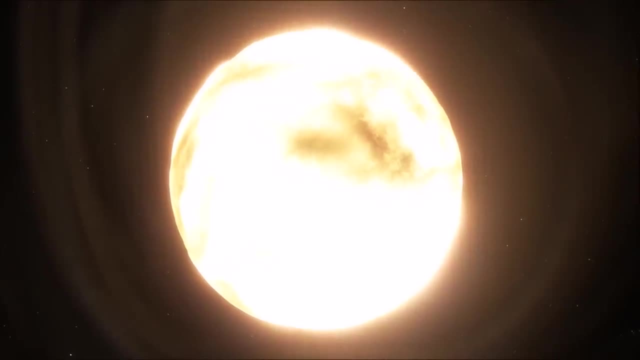 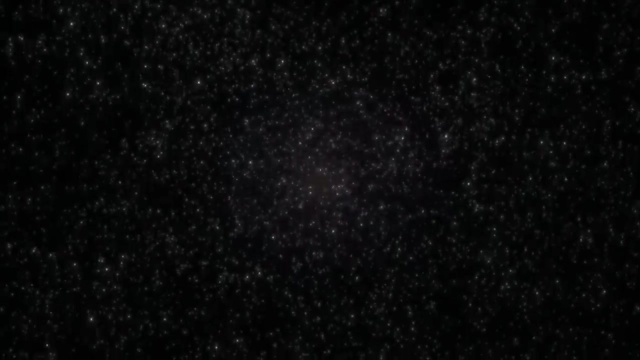 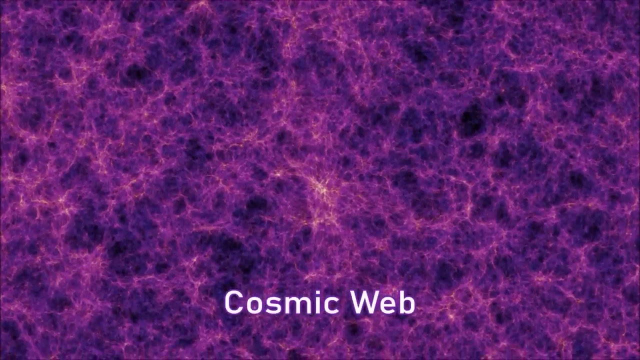 have become stars And today most of those stars belong to enormous ancient galaxies. Most of these galaxies are gathered in large clusters and superclusters which all connect to form a 3D path across intergalactic space, known as the cosmic web. When we talk about space, most of the time 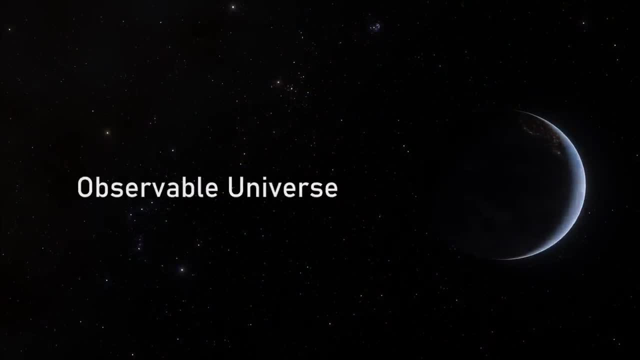 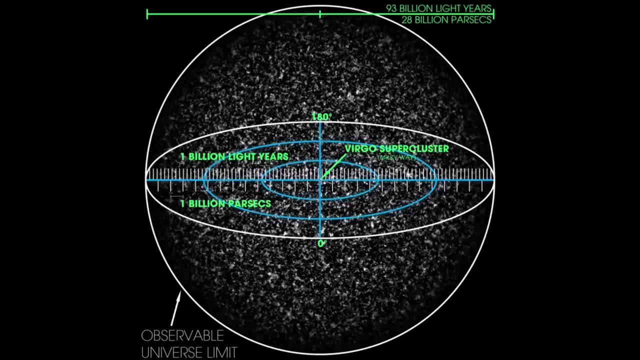 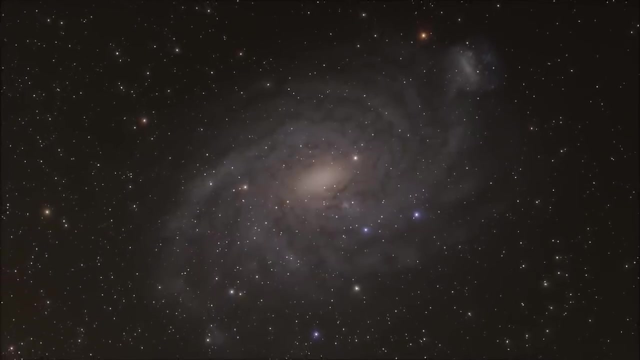 we are referring to the observable universe or the known universe. This is a spherical, geocentric region of space. It is comprised of all the galaxies and matter that can be detected from Earth because their light emissions have had enough time to reach the solar system since they were emitted. 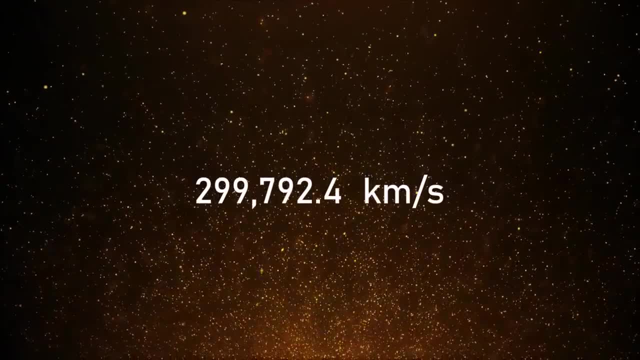 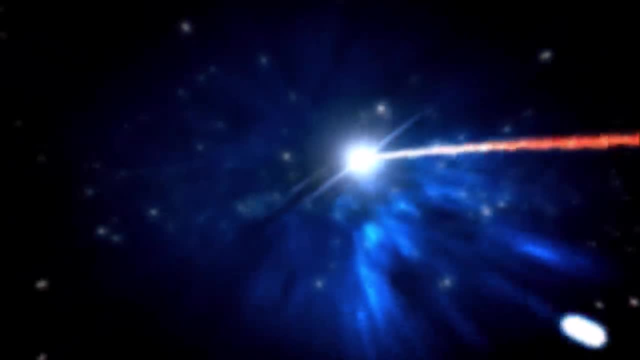 Light travels at just under 300,000 kilometers per second. That is extremely fast, the fastest speed attainable in the universe, in fact. But even just beyond our galaxy there is a light delay which impairs our ability to see the universe as it appears now. 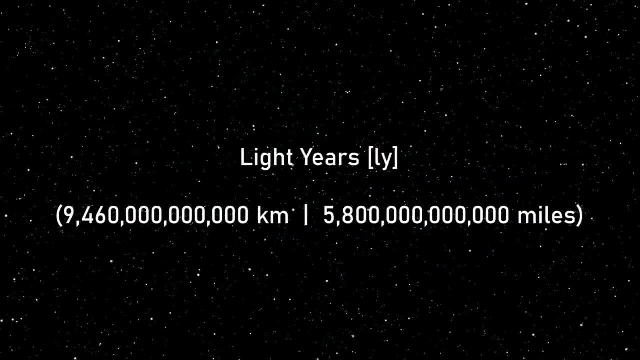 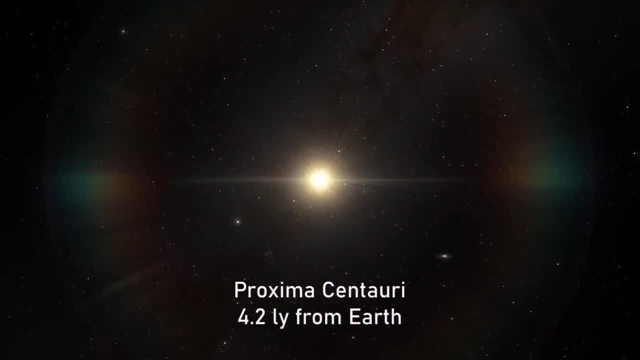 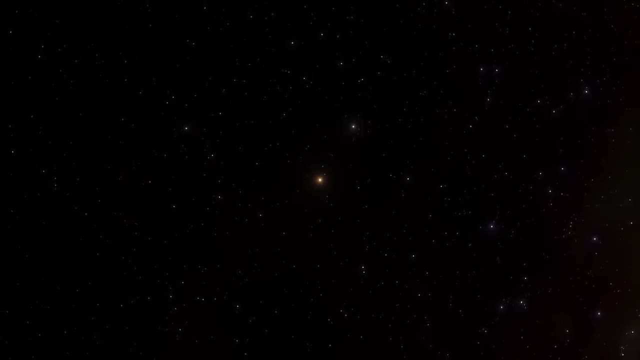 That's why it helps to use light years as a unit of measurement. Proxima Centauri, our nearest star, is 4.2 light years away, meaning we see the star as it was about 4 years ago, and that's just on a stellar scale. The space between galaxies is incomparably larger. The distance between us and our nearest spiral galaxy, Andromeda, is around 2.5 million light years. we see Andromeda as it was when humanity had only just started using stones as tools. The further away a galaxy is, the longer the light travel time and the younger the galaxy appears to. 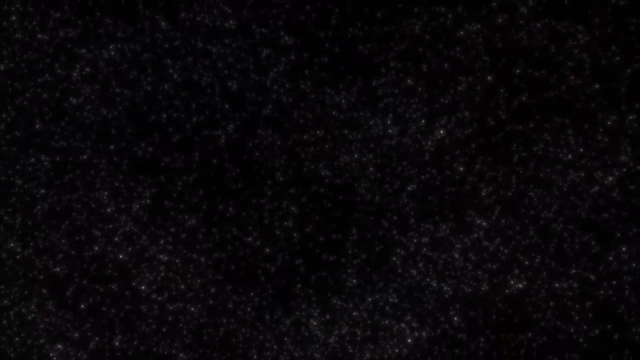 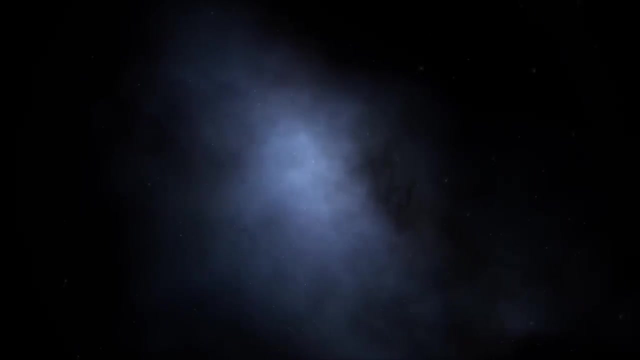 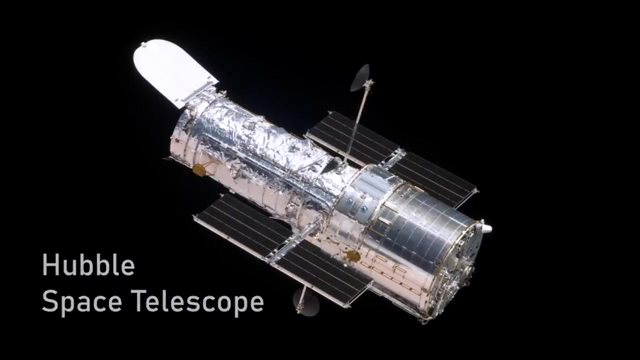 be, And so the deeper we look, the further back we are looking in time through the different stages of the universe's life, And nothing has allowed us to look deeper into this rich history than the magnificent Hubble Space Telescope. The Hubble Telescope is a bus-sized satellite. 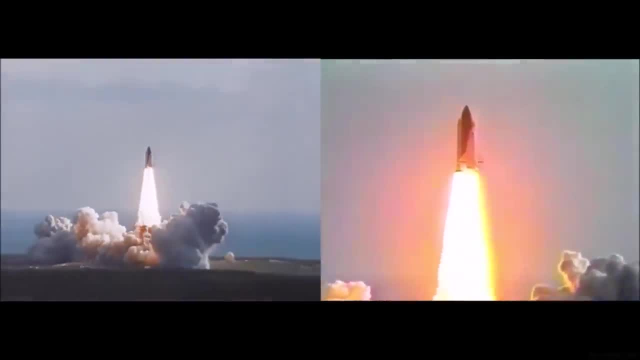 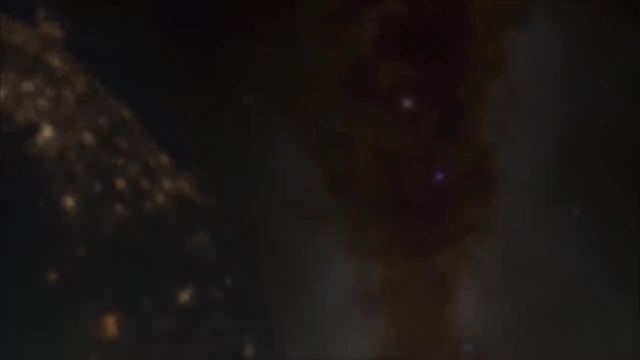 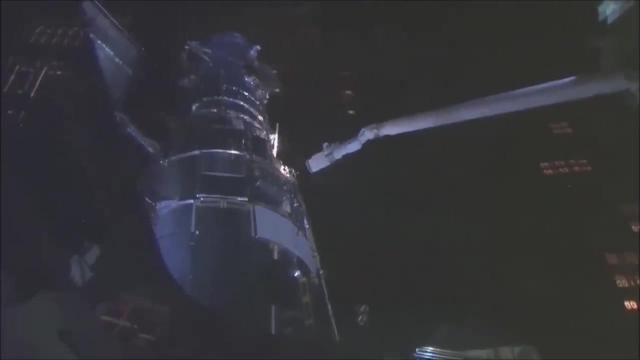 which launched in 1990.. It orbits the Earth and faces out towards space, allowing it to image the universe undeterred by atmospheric disturbances which hamper ground-based telescopes. It has a number of different instruments and filters and has received numerous upgrades throughout the 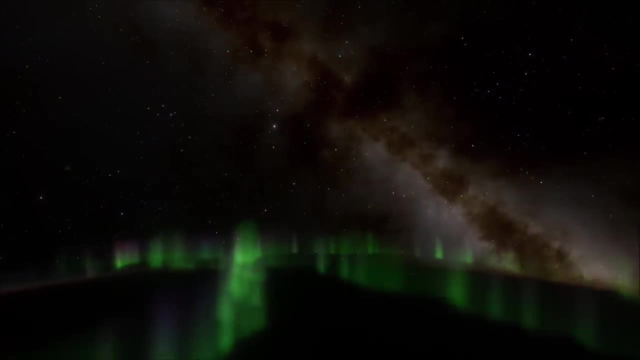 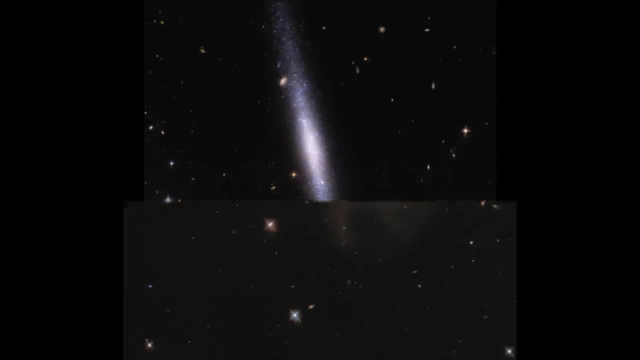 years, which have kept it up to date. The Hubble Space Telescope is the largest space telescope at the forefront of human technology. Hubble has snapped over 1.1 million bedazzling images of the cosmos since its launch, from nearby stars and nebulae to galaxies at the very distant edge of 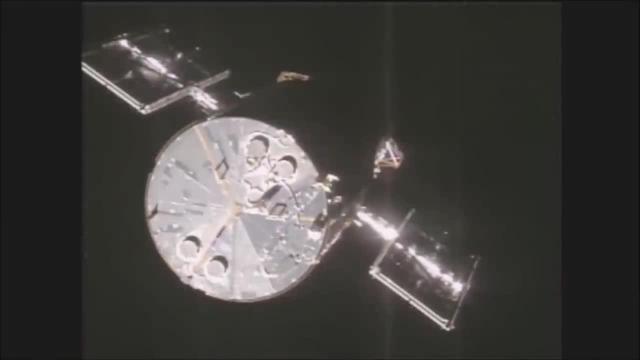 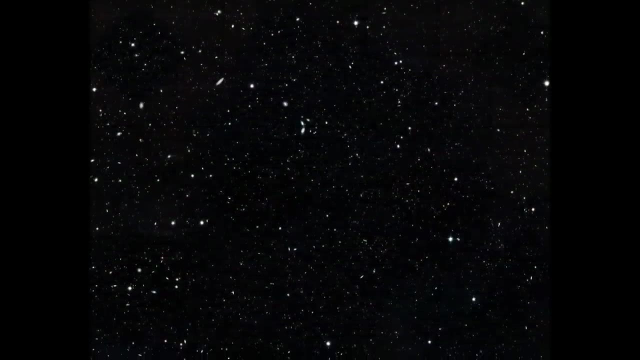 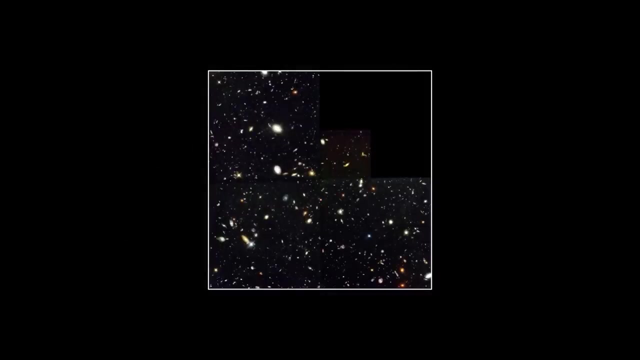 the observable universe. Its deep camera technology allows us to look ever deeper into space, revealing a much younger universe that has been constantly changing and evolving. Nothing captures this evolution quite like the Hubble Deep Field. The Hubble Deep Field image is one of the most important images ever. 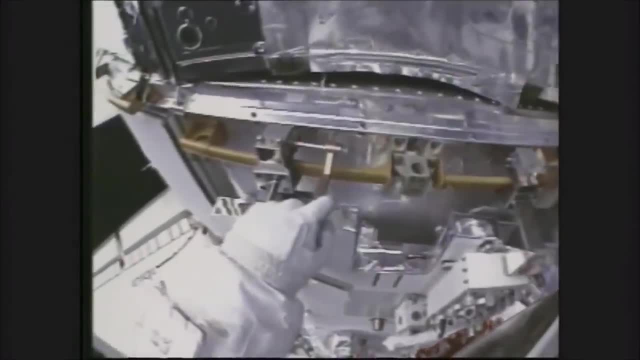 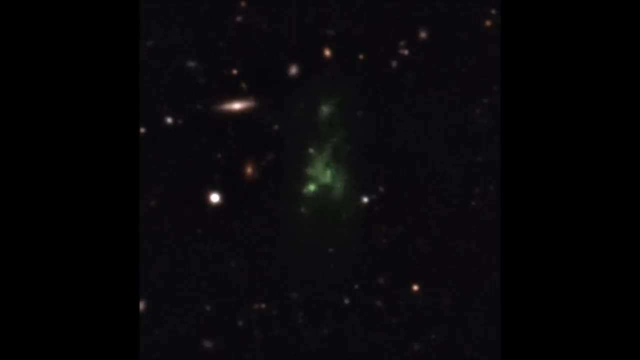 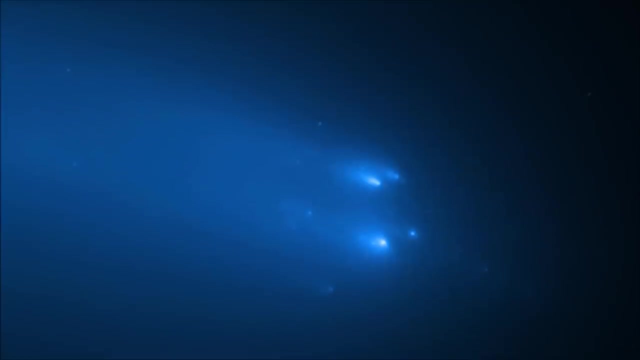 It was taken in 1995 after Hubble received a servicing upgrade two years earlier which dramatically broadened the telescope's ability to see the most distant galaxies. Around one tenth of the Hubble Telescope's operational time is allocated to high-ranking staff and physicists wishing to study unexpected phenomena. 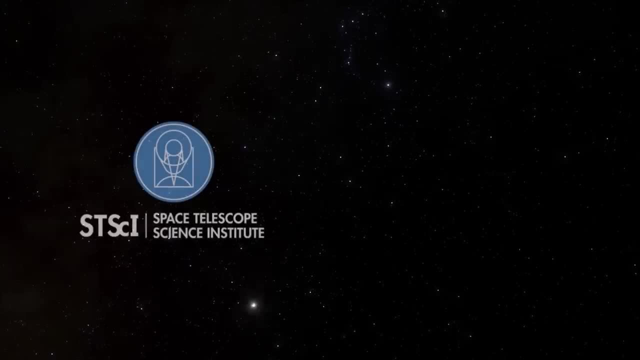 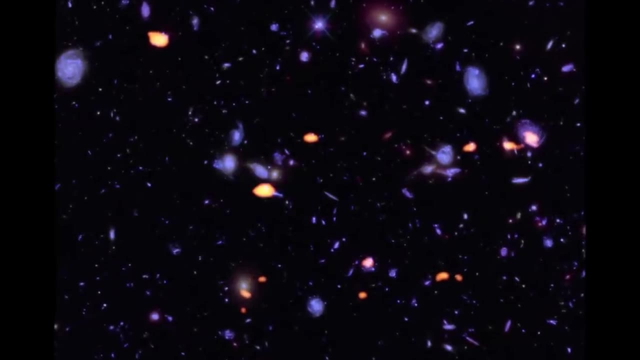 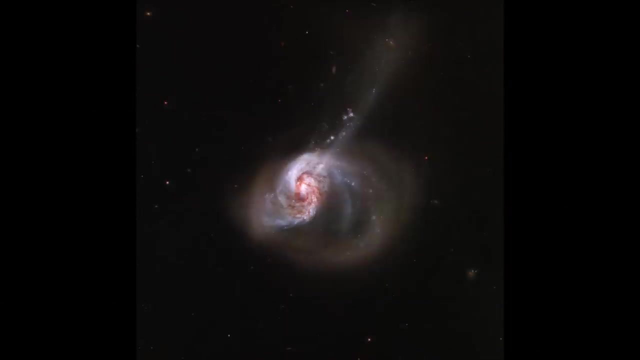 And so the then-director of the Space Telescope Science Institute, Robert Williams, devoted his time slot to imaging extremely faint and distant galaxies as a means to test our theories on the age and size of the universe. Unlike most of the images captured by Hubble, which usually have a luminous target, the Deep Field, 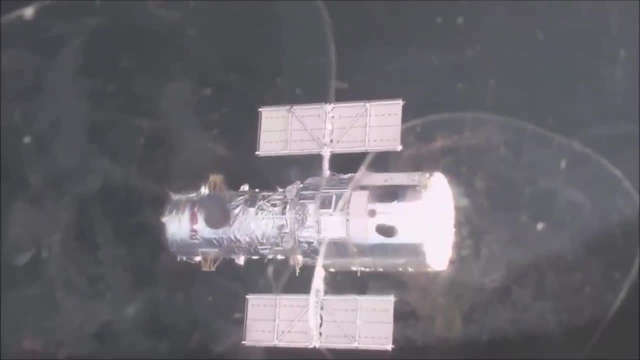 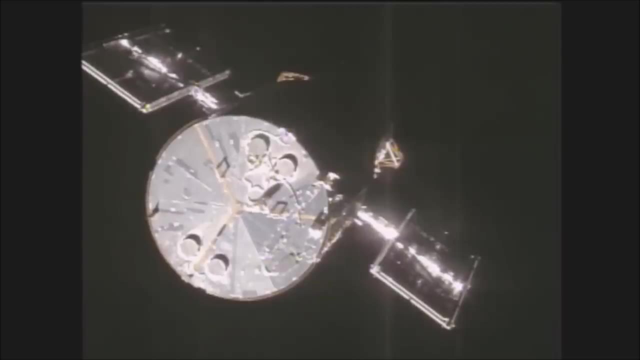 Image was created by focusing the telescope's instruments on a tiny, seemingly empty patch of the night sky where nothing can be seen from the Earth. In order for this to work, the telescope needed an area with a high enough galactic latitude that the field would not be obscured. 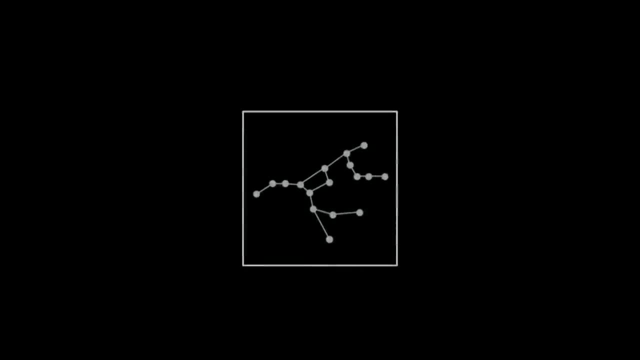 by the light from the Milky Way's core. Thus, a small area was chosen in the constellation of Ursa Major, also known as the Big Dipper or The Plough. The point chosen by Williams in the video that you can watch in the video description is at the top of the Ersa Major of the PETA. 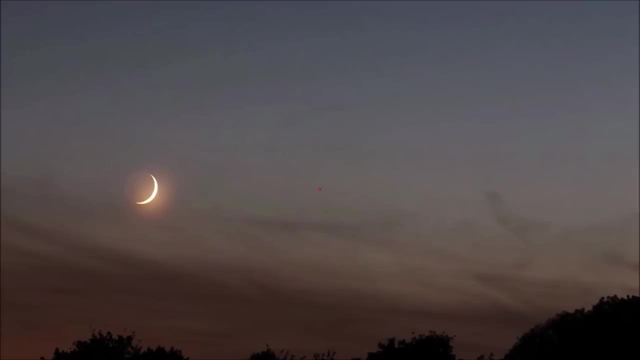 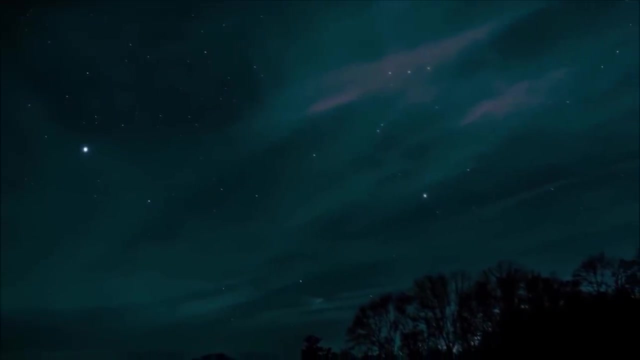 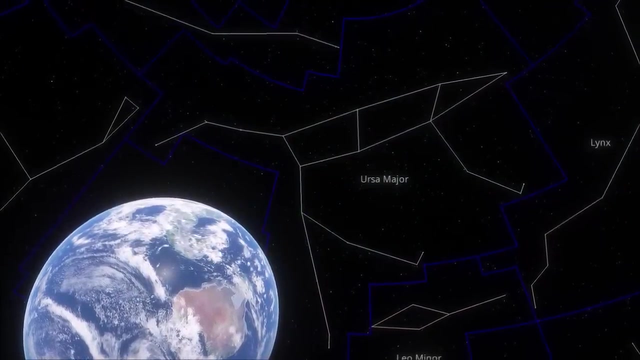 The point chosen by Williams was tiny- an area roughly 1, 12th of the diameter of the Moon in the sky, equivalent to a mere 1, 24 millionth of the total night sky expanse. Over some 10 days, the telescope gathered light from the area and 342 photographs were taken using a variety of 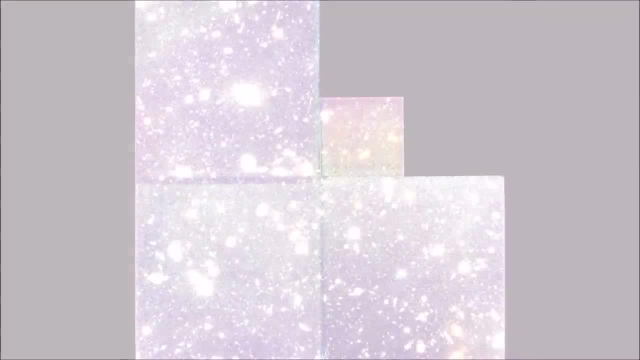 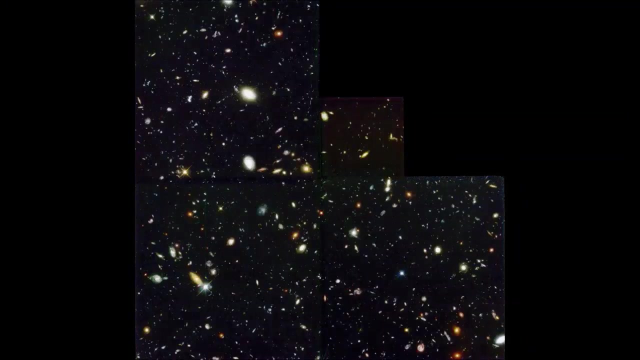 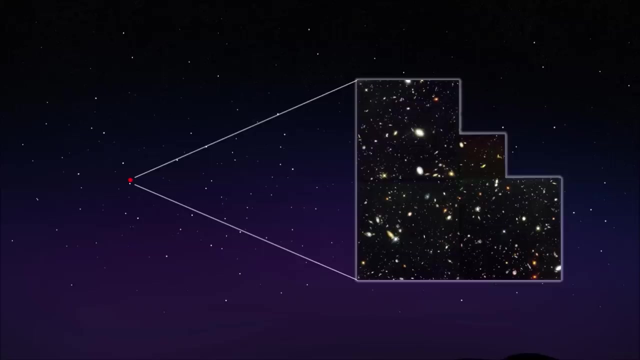 the telescope's filters. The data was then processed and the image was compiled, revealing a majestic view of the universe's history. Contained within this tiny, pin-sized segment of the sky are over 3,000 galaxies at an array of distances, including some of the oldest and 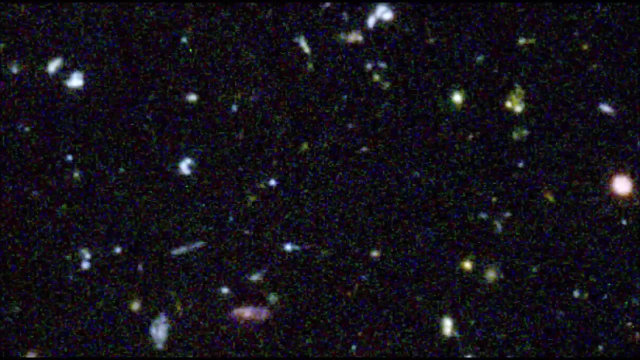 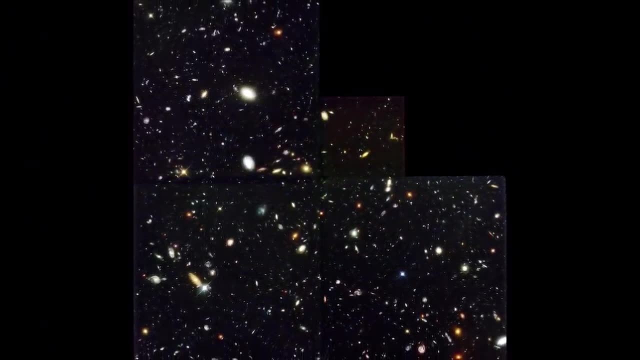 most distant that had been discovered at the time. This image isn't so much a representation of distance in the universe- rather, it is a window back through time. In the shallower field, we can see rich spiral-glazed images of the universe, and we can also see rich spiral-glazed images of 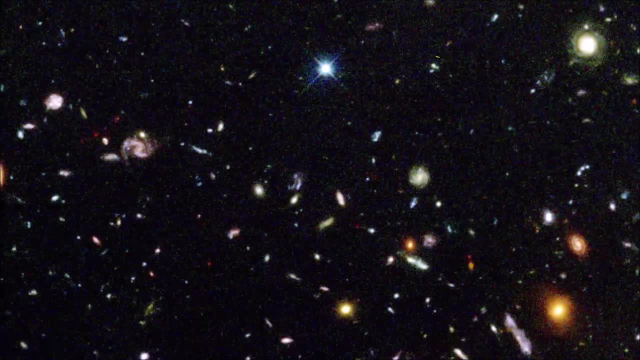 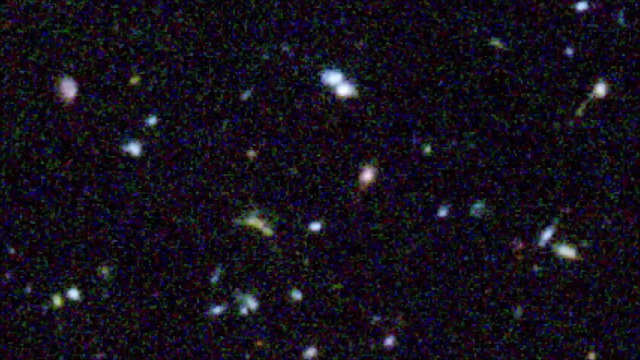 galaxies, But the further back we travel, the less luminous and structured the galaxies become. Most of the very distinct galaxies in the image occupy only a few pixels and shine much less brightly, because these early galaxies had not had much time for vigorous star formation. 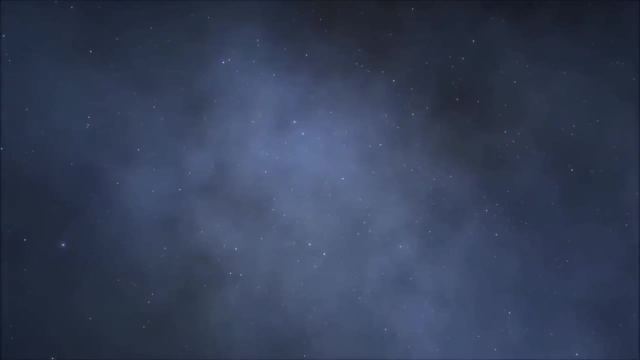 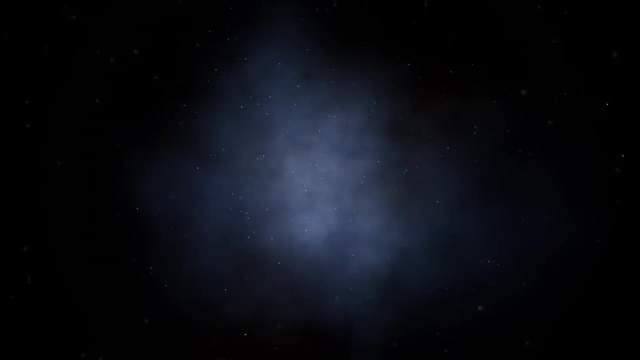 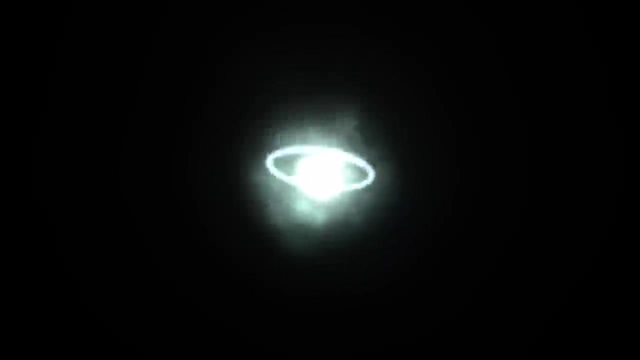 but instead had lots of early star-forming gases. The presence of many unstructured, irregular galaxies in the early universe reaffirms our belief that- After the big bang, matter began building around the world from the ground up: First atoms, then stars, then clusters of stars, then Taurid, dwarf galaxies- Which is why a net 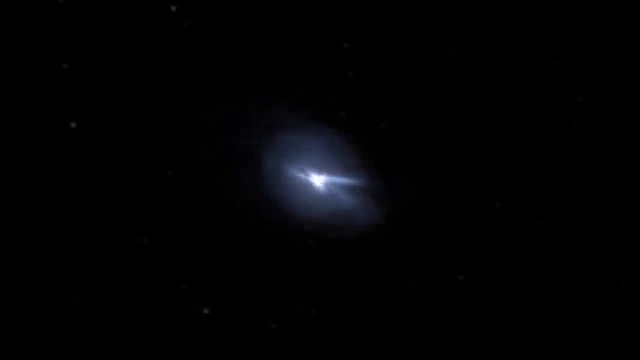 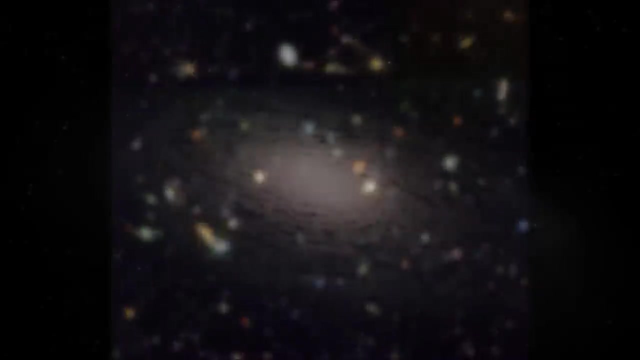 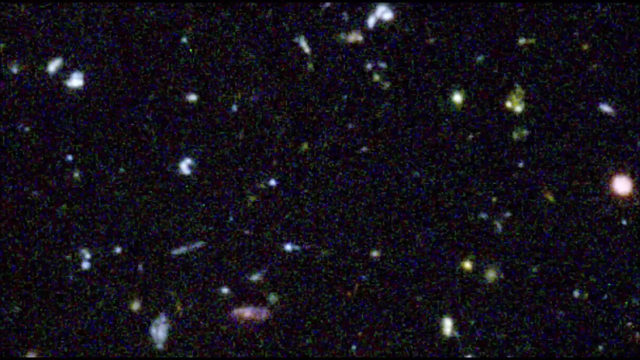 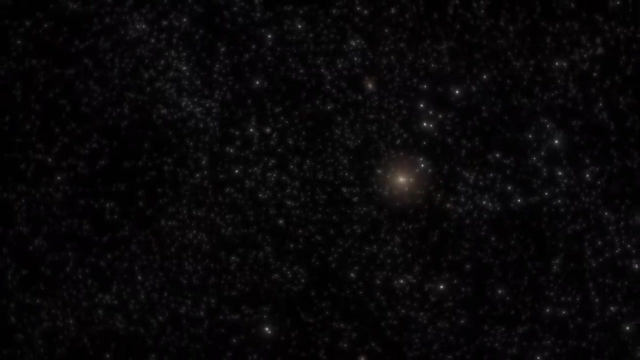 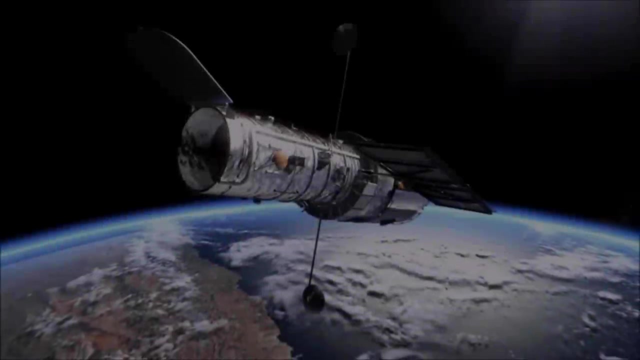 hit starts building up, causing numerous galaxies to collapse, as it is today, then we would probably see large spiral and elliptical galaxies like we do in our surrounding space. But again, light just gives us that special opportunity to stare backwards through time. 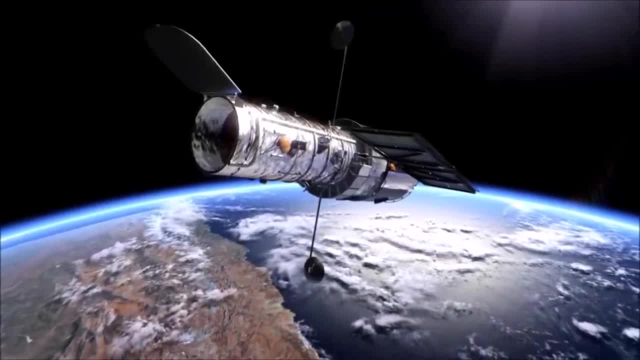 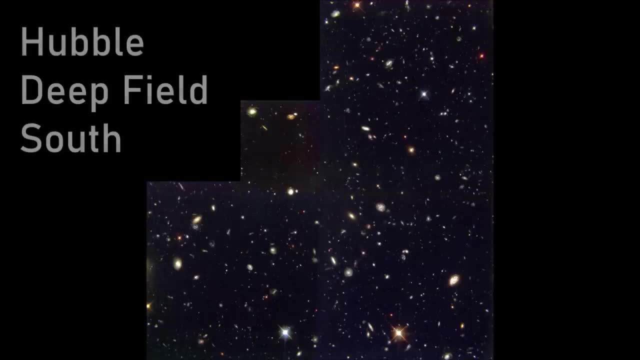 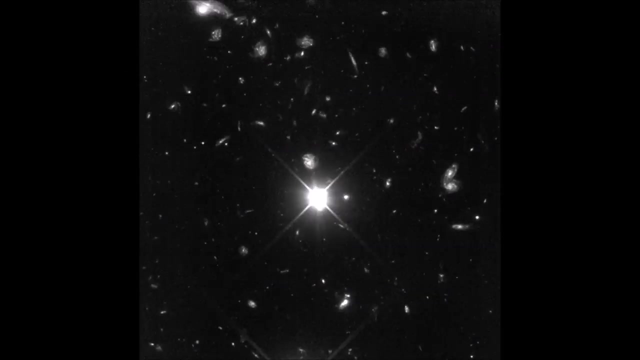 In the following year, a follow-up Deep Field image was taken to ensure that the original was truly representative of the distant universe. The results of the Hubble Deep Field South image were much the same this time, even capturing the light from a quasar in the early universe. 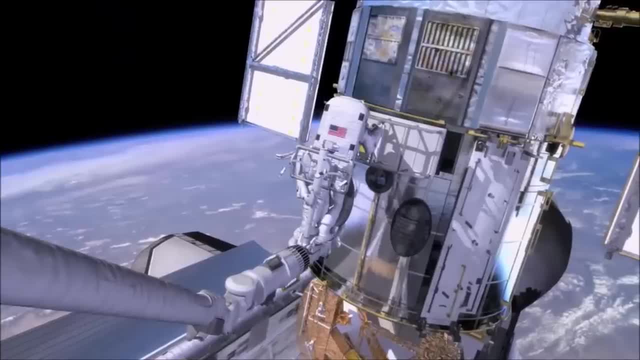 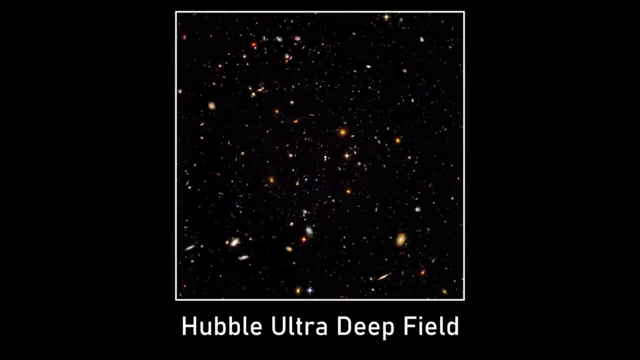 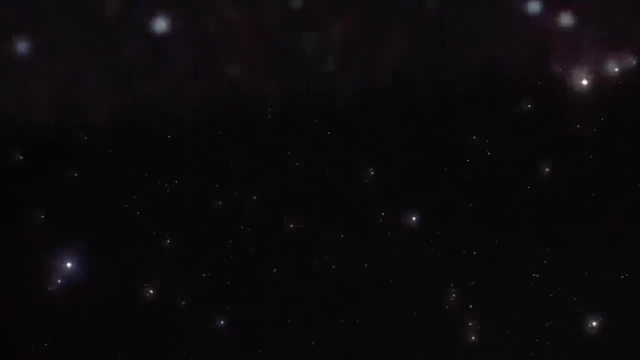 After another servicing mission to Hubble in 2002, the telescope was able to take even deeper images still, and in 2004, they snapped the Hubble Ultra Deep Field, the deepest photograph of the universe ever taken from the constellation of Fornax. This image reaches the limit of 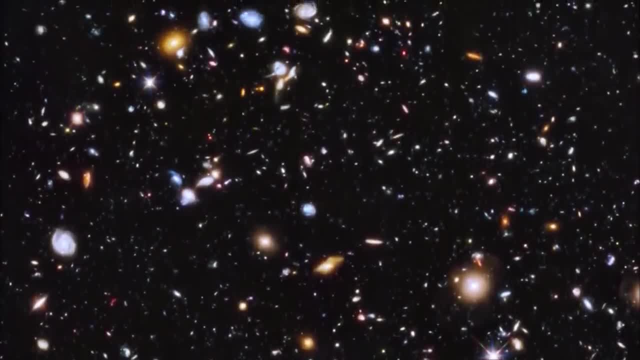 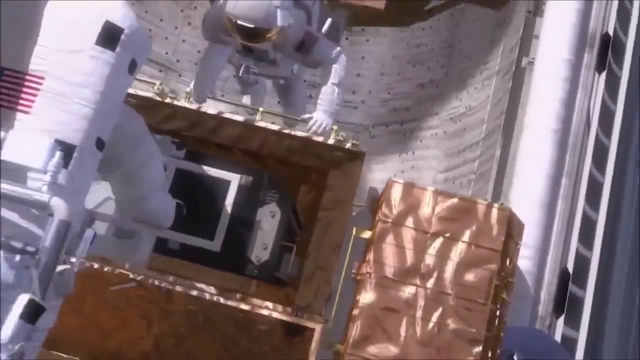 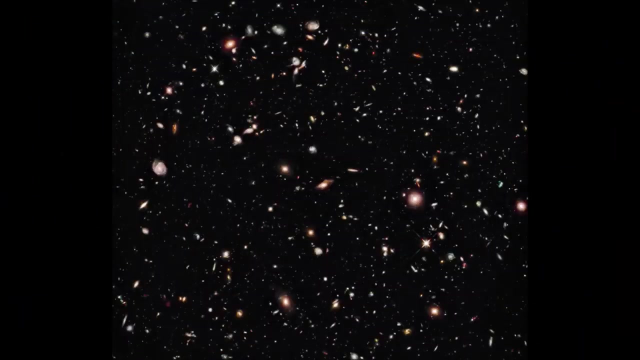 what is possible to observe. To see any further back, we need to use infrared radiation. A 2009 servicing mission to Hubble equipped it with new sensitive infrared detecting instruments, and Hubble re-snapped all three deep fields in infrared, this time revealing thousands more primordial galaxies and several. 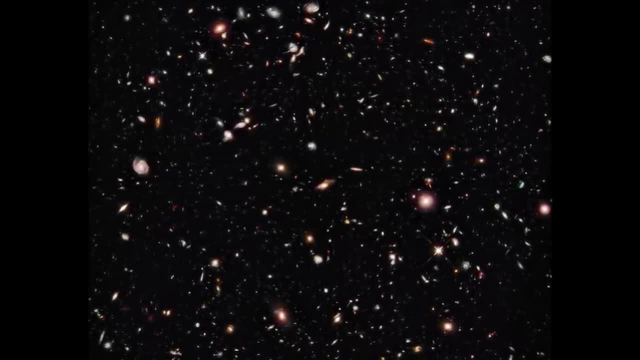 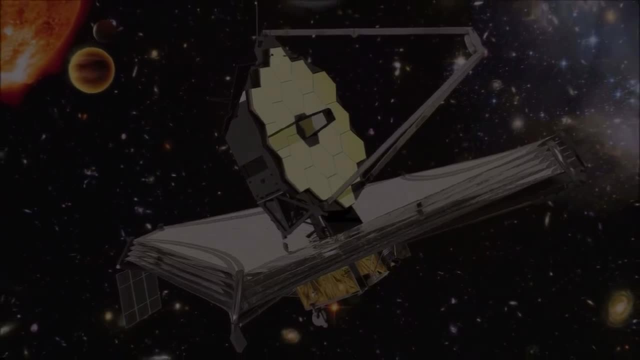 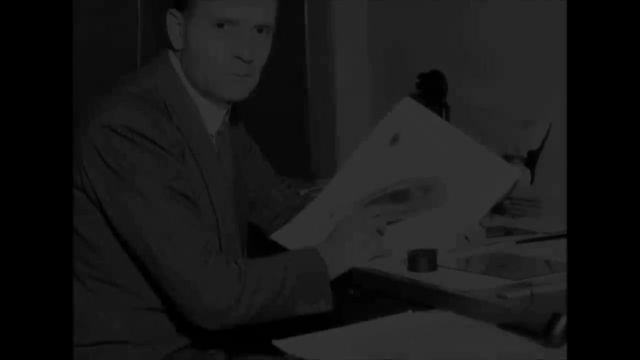 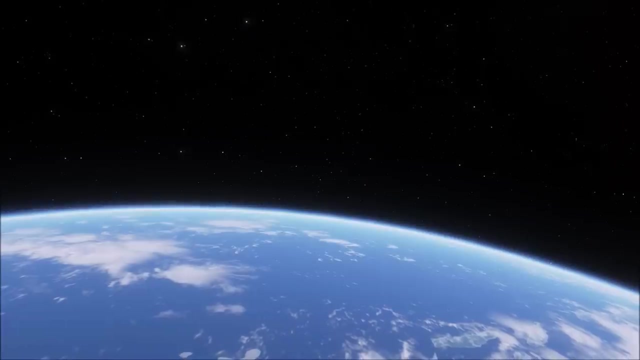 of the most distant ever to be observed, And we probably won't get a better picture than this one until the James Webb telescope finally launches. Edwin Hubble and his accompanying legacy have had a profound impact on modern day astronomy, But of his discoveries one sticks out from the rest, underpinning everything. 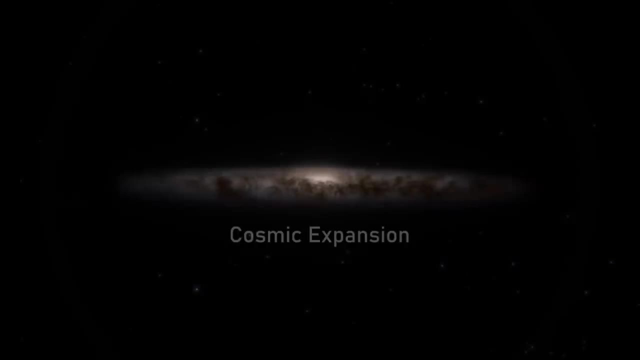 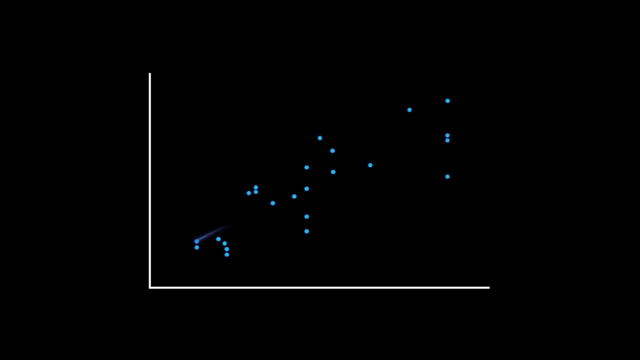 that we observe and have spoken about today: Cosmic expansion, The discovery that the universe itself is expanding, The discovery that the universe itself is expanding. This came about after Hubble had surveyed 24 newly discovered nearby galaxies and had established a linear relationship between the radial velocity of the galaxies and their 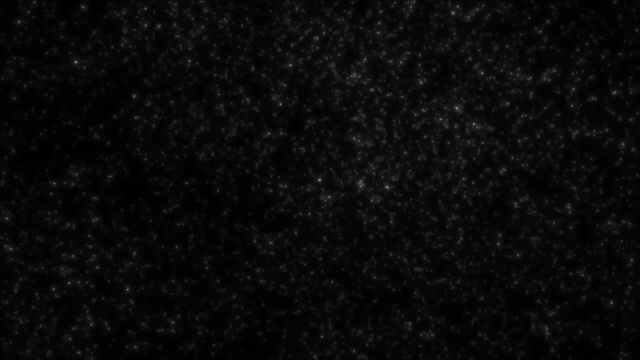 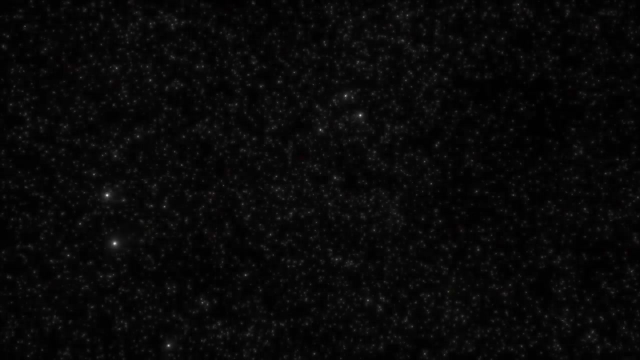 distance from Earth. Simply put, galaxies outside of our local galactic group all appear to be moving away from us, and the further away they are, the faster they appear to be receding. Everything in the universe seems to be moving away from everything else into. 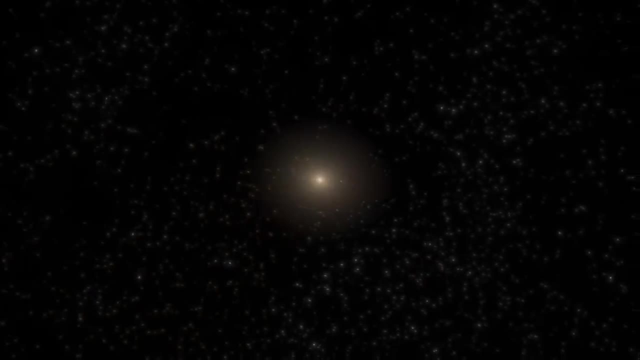 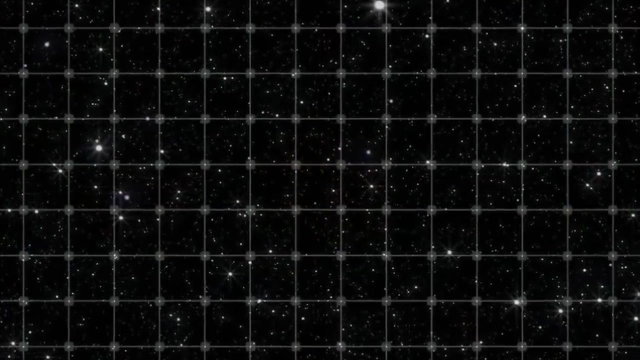 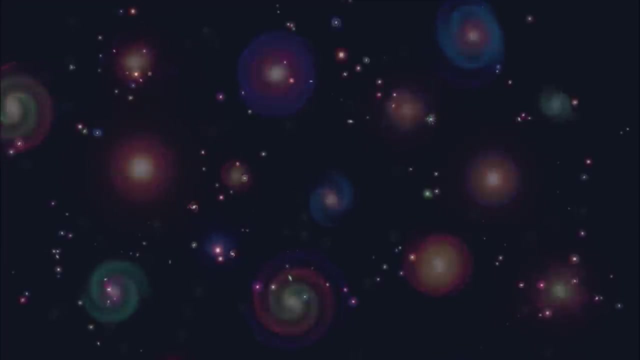 its own pocket of space Without changing its position. Hubble's conclusion was that space itself is expanding at a consistent rate across all points, spreading the galaxies of the Universe further apart from each other. When space expands, new space is created everywhere, all over the universe Space itself stretches. 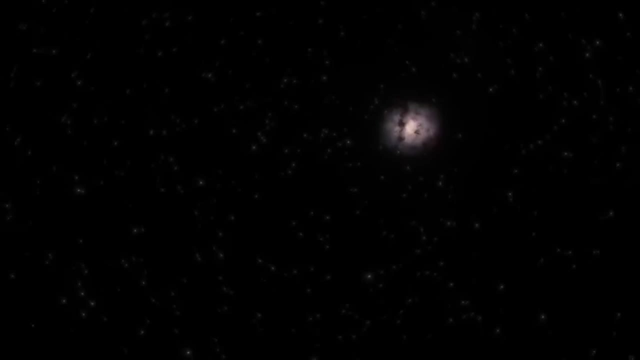 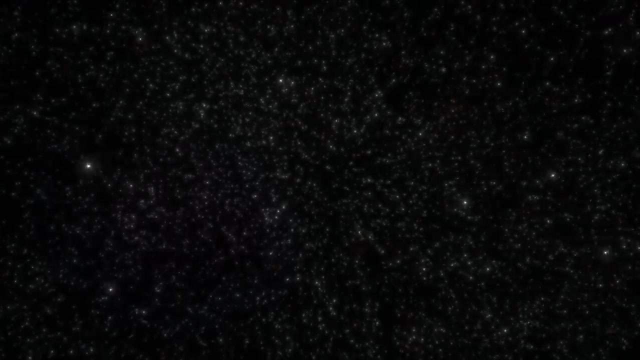 apart in every direction to make more space. It is like the universe is inflating rather than expanding. See no other opposed to the universe. space itself stretches apart in every direction to make more space. it is like the universe is objects are getting further away from all other objects relative to each other. there 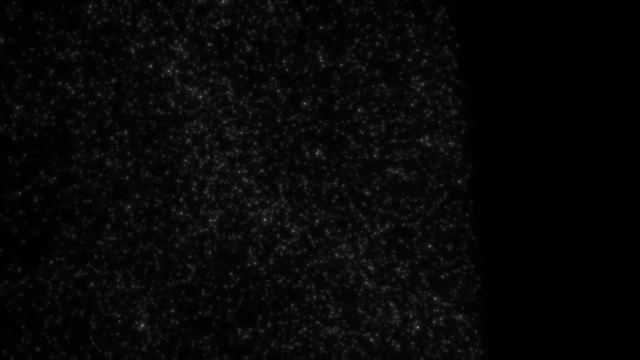 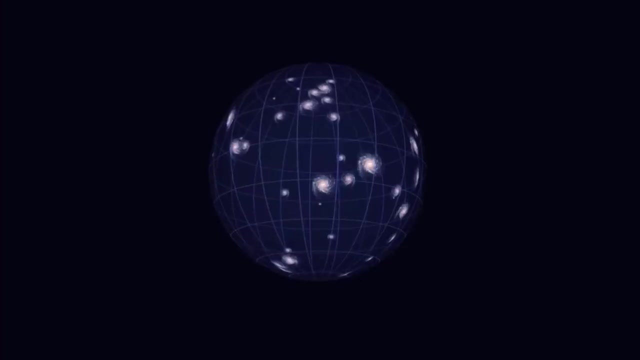 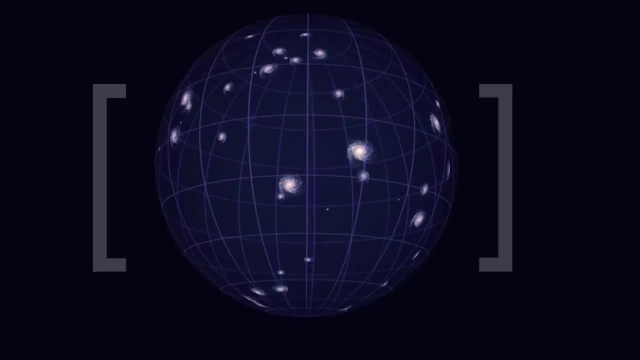 is no centre Space has no boundaries, edges or walls that mark the end. So how do we go about visualising this? Well, imagine that this sphere represents the universe, but rather than space being on the inside, it is mapped to the outside surface As the sphere expands. 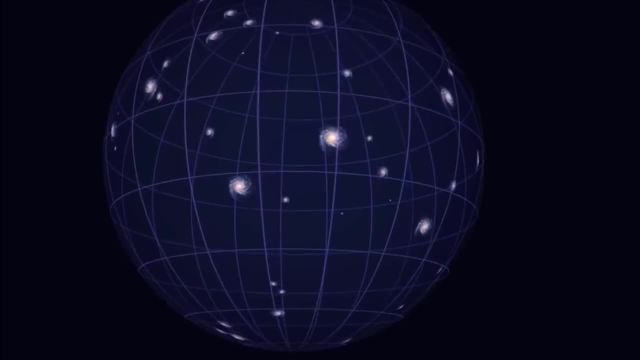 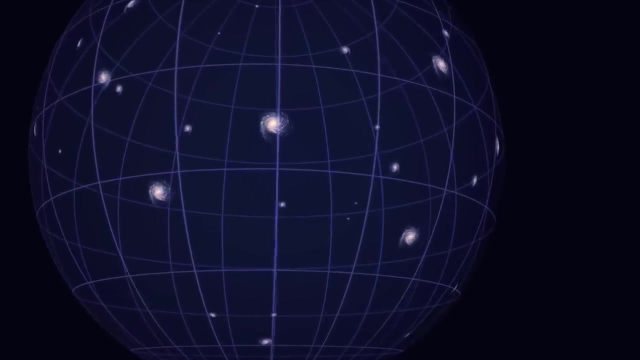 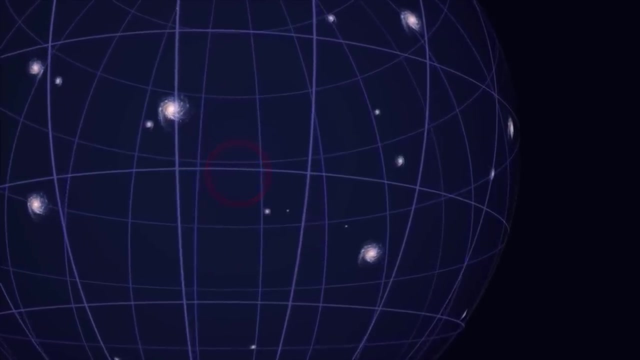 the surface area of the space for the outside galaxies increases at the same rate and, as such, there is no centre. No galaxy on this sphere's surface is any more central than any other galaxy. Of course the sphere itself does have a centre, but this doesn't represent 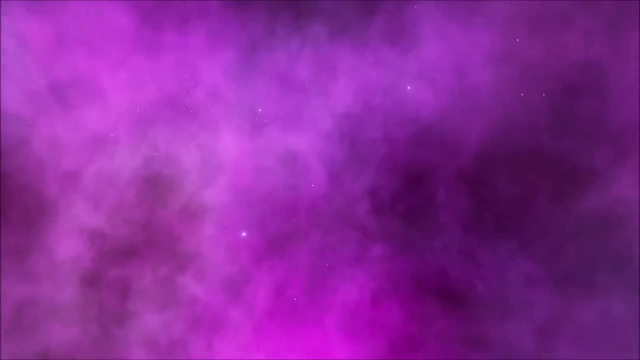 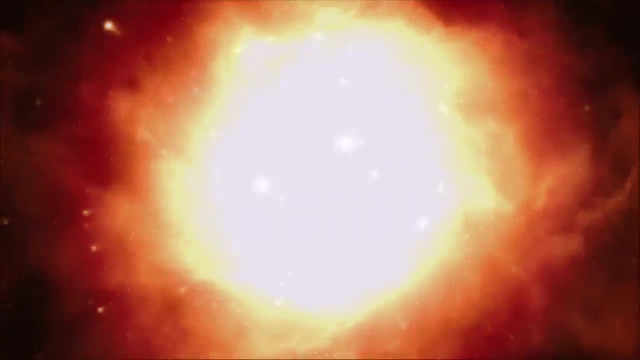 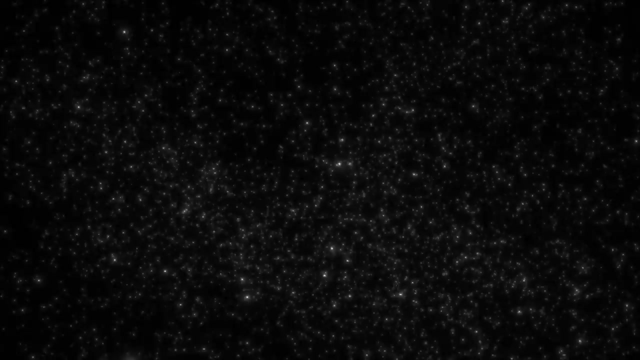 a physical location within the universe. Rather, it represents a point in time, The big bang. It's an odd concept, but what this means is that, even if space is finite and only occupies a certain volume, you could still roam around the universe indefinitely. 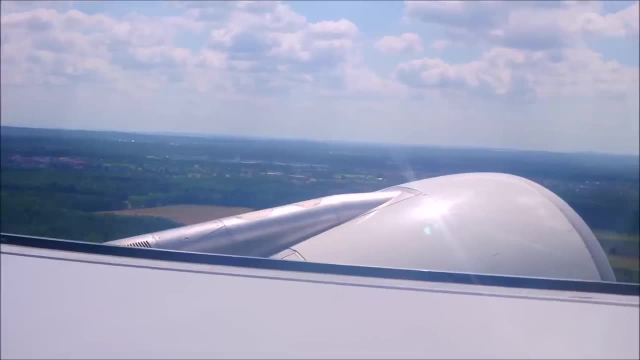 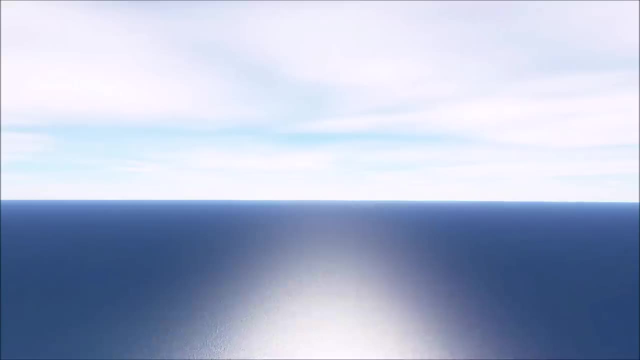 without meeting an edge, Much like if you were to fly an aeroplane round the Earth's equator. you would never fall off or run out of Earth to fly across. Instead, gravity would just bring you back round to the same place eventually. So if you were able to travel, 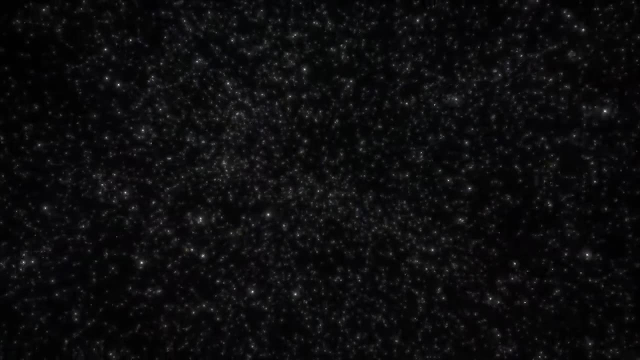 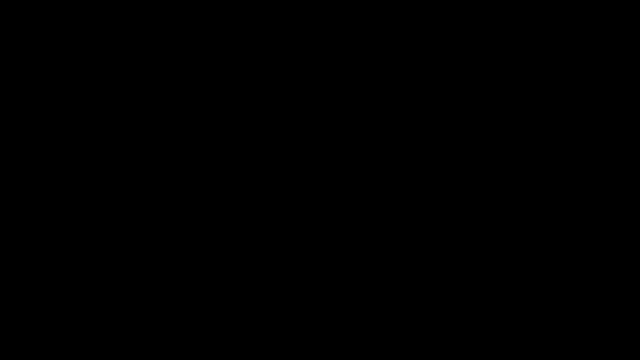 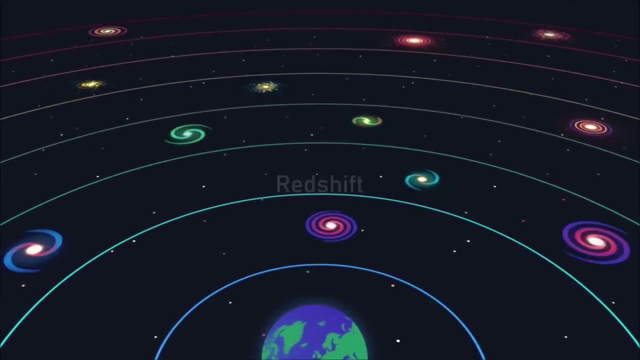 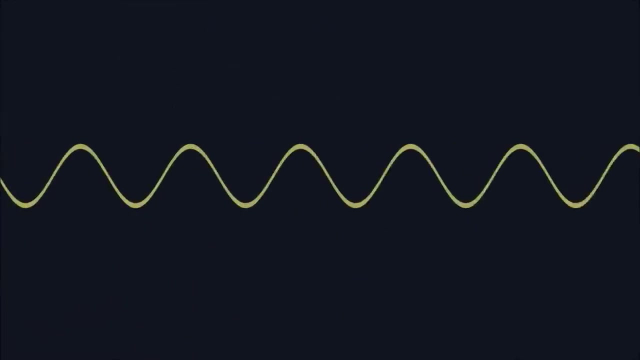 considerably faster than light speed. in a straight line, you would still come back to the same place. eventually. We can see evidence of the universe's expansion everywhere, thanks to a phenomenon known as redshift. Redshift is when electromagnetic radiation, such as visible light, undergoes an increase in wavelength. The wave is stretched. 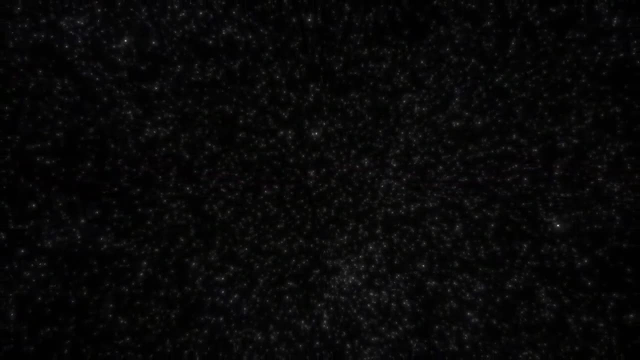 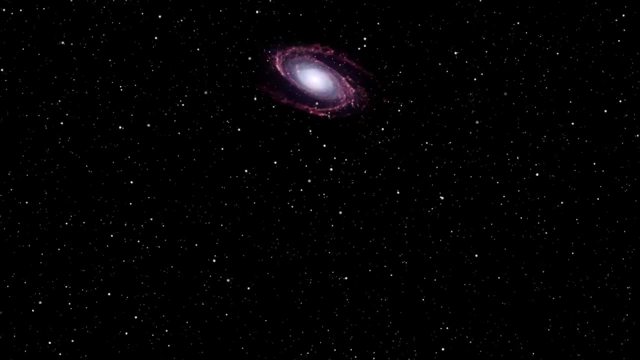 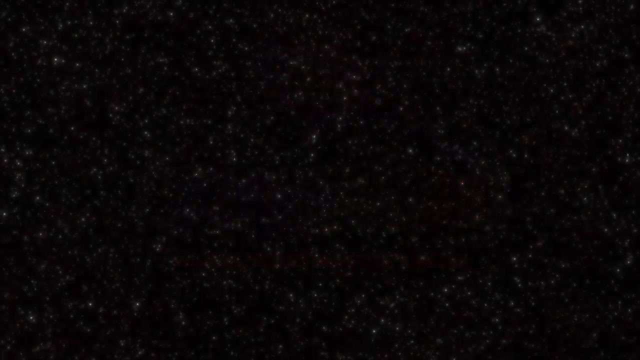 out, resulting in a decrease in wave frequency and photon energy For visible light. you would need to have a radio wave. You would need to have a radio light. When analysing a galaxy's spectral emissions, this has the effect of shifting the absorption lines of certain elements towards the red end of the spectrum, turning visible. 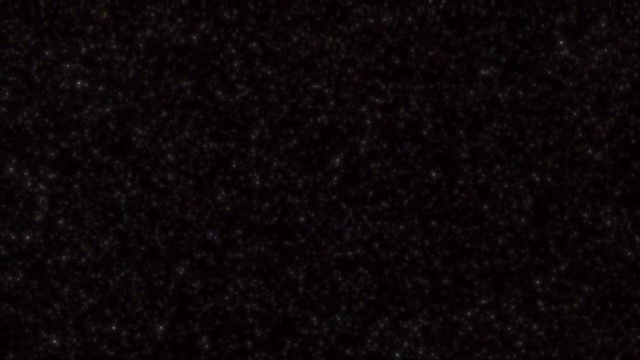 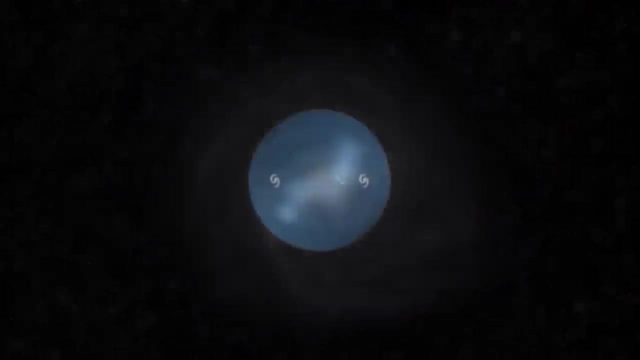 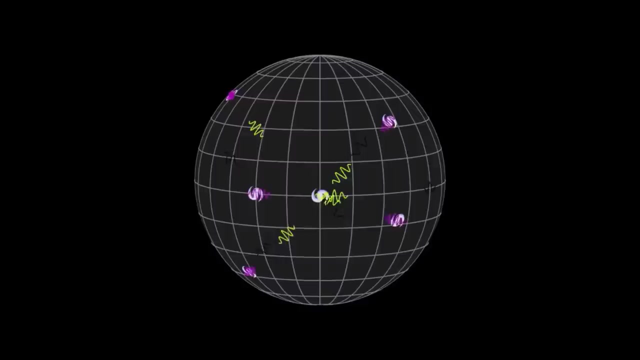 light red Because the universe is expanding at all places at once. as the light emitted from other galaxies travels towards Earth, the space it travels through elongates, stretching out the waves and redshifting the light. The more distant the galaxy, the further a. 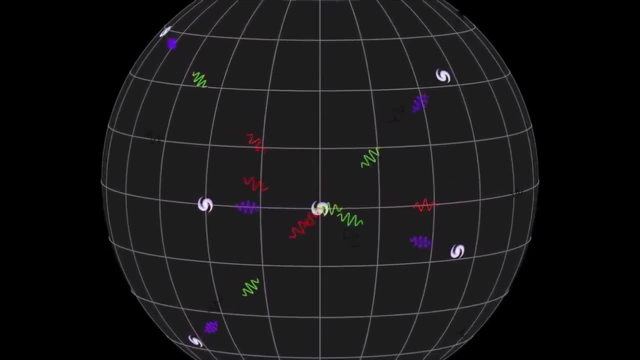 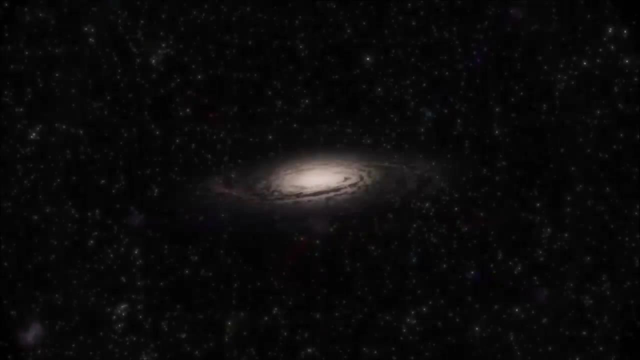 cross ever-expanding space. the light has to travel, and so light from more distant objects is redshifted more, And we can use this to determine how much the universe has expanded since said light was emitted. The Hubble Constant, a measure for the rate. 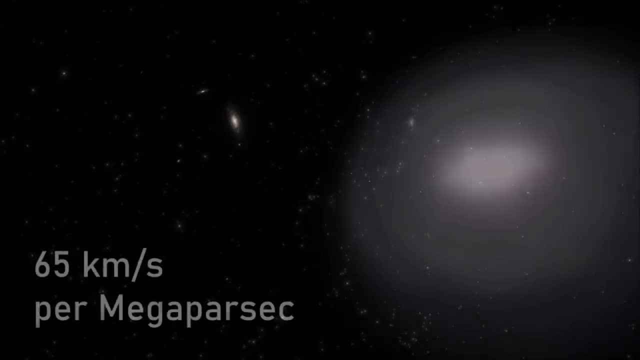 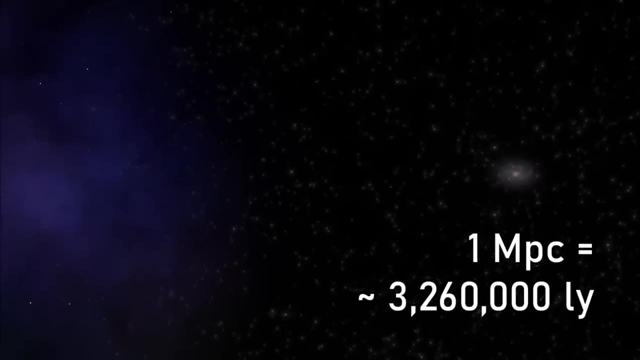 at which space is expanding is thought to be around 65km per second per megaparsec. A megaparsec is equivalent to about 3.2 million light years, So the more megaparsecs there are between us and a galaxy, the more light we can emit. So the more megaparsecs there are between us and a galaxy, the more light we can emit. So the more megaparsecs there are between us and a galaxy, the more light we can emit. So the more megaparsecs there are between us and a galaxy, the more space there is between. 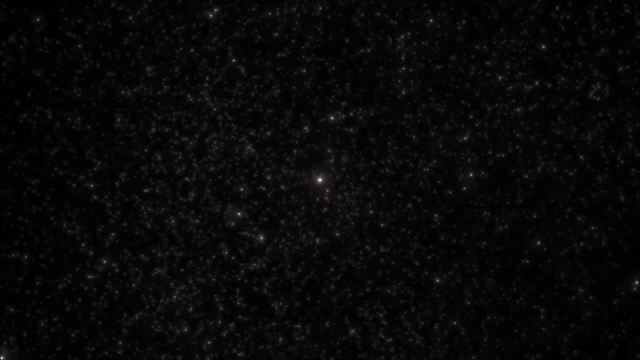 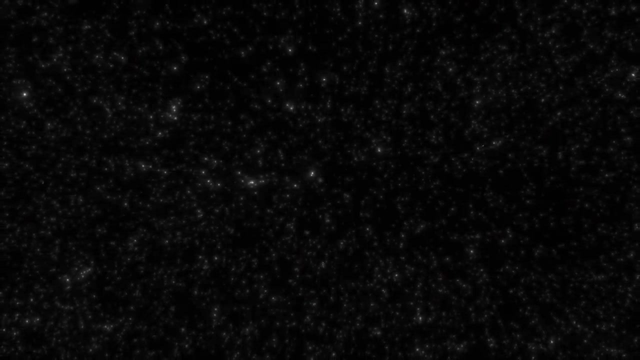 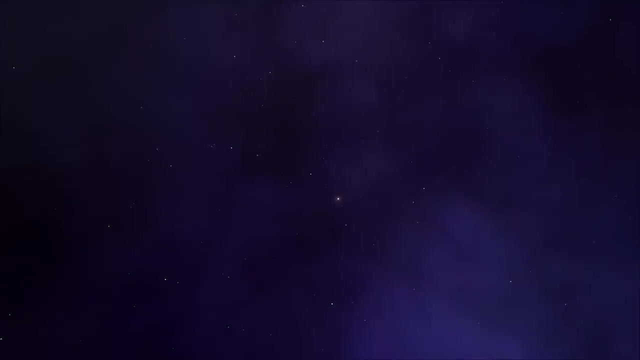 the two. that is expanding, causing the galaxy to recede away faster. For example, 100 megaparsecs away, the space is receding away from us at a rate of over 6,500km per second. Because light speed is limited to about 300,000km per second, there eventually comes a distance. 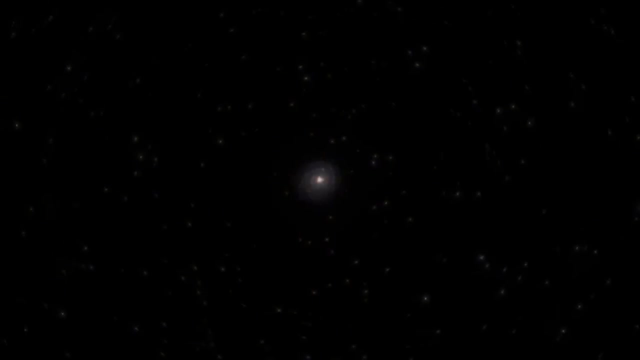 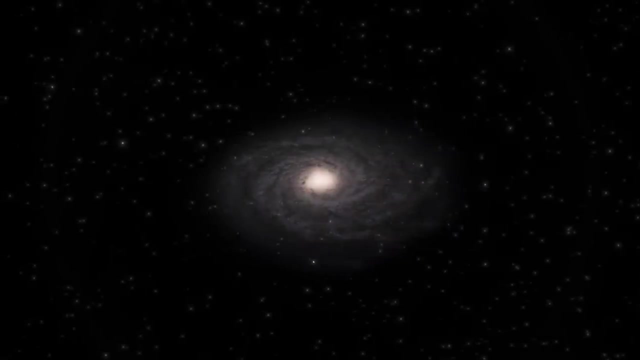 from the Earth, at which galaxies are being pushed away from us faster than light speed, Not by breaking any laws of physics, because they themselves are not moving that fast, but because there is simply too much space between us and them for their light to be. 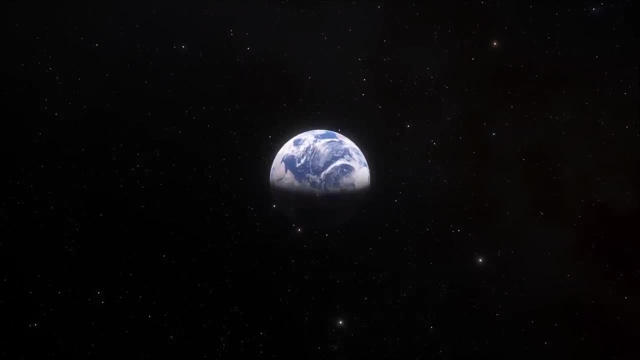 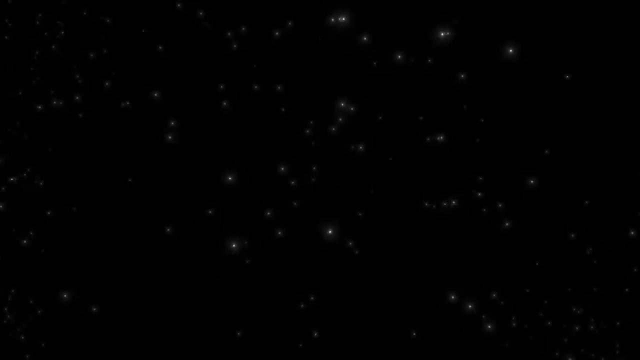 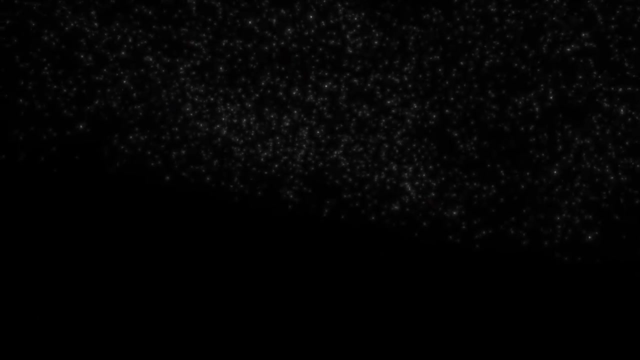 able to cross the universe in time to reach us. This constitutes the edge of our observable universe, the boundary beyond which we are unable to see any further, The Cosmic Horizon or the Particle Horizon. Before this boundary, light from the Cosmic Horizon would have been. 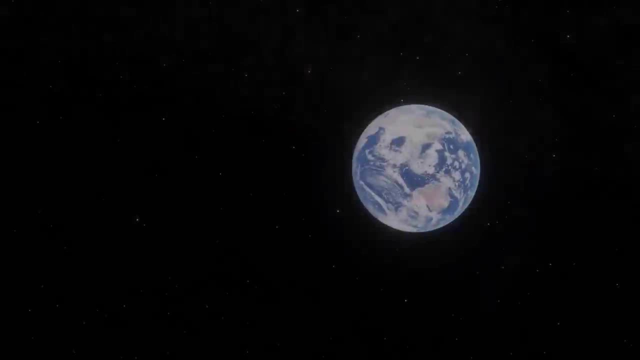 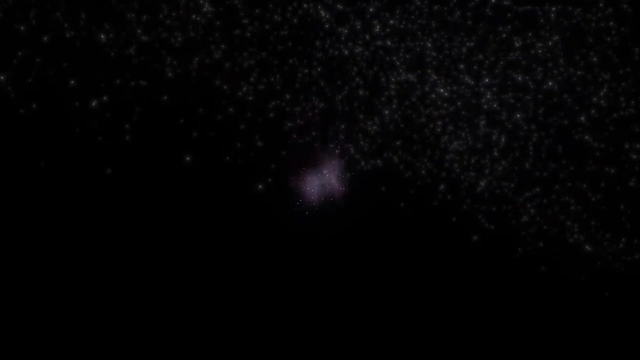 a very distant galaxy. but the light from distant galaxies has had enough time to cross the expanding universe and meet our telescopes. But beyond the Cosmic Horizon, the light from the galaxies has either not had enough time to reach the solar system or it is so far. 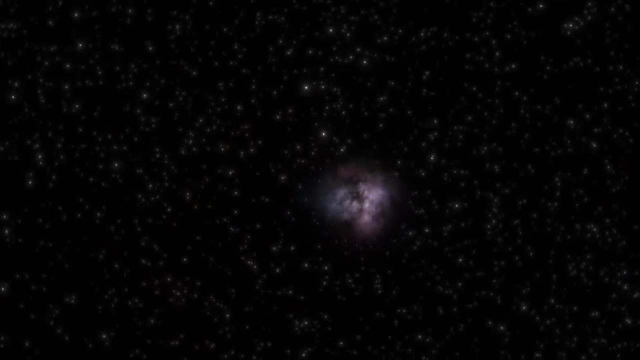 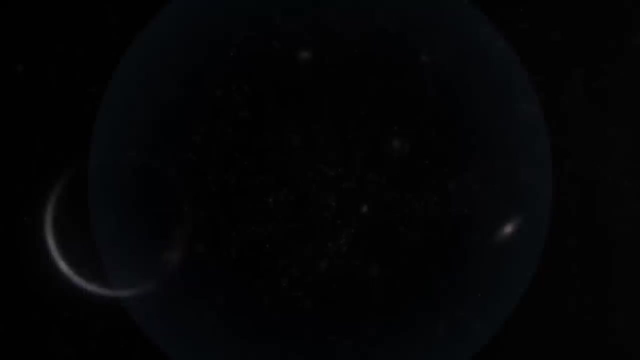 away that it will never be able to reach the solar system. As time passes, older and more distant light has time to pass through the solar system and the observable universe grows, increasing our field of view, But this is entirely dependent on the distance between 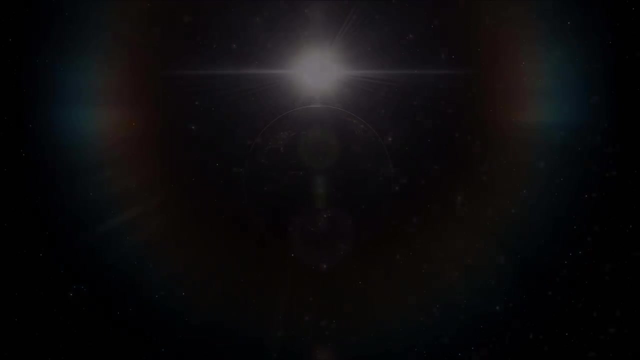 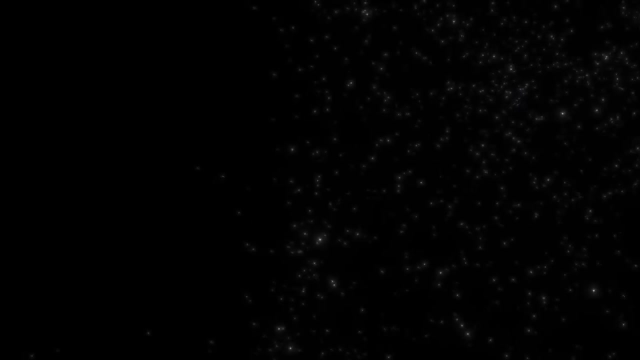 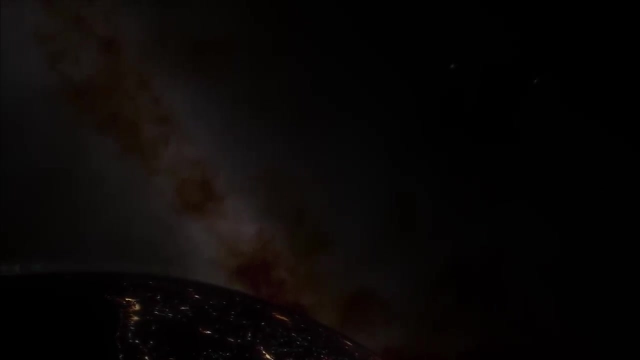 us and the Cosmic Horizon. For an observer at the Cosmic Horizon, space would appear much the same, But relative to us. space beyond the Cosmic Horizon is what's known as causally disconnected, Unreachable and undetectable to us by any known means. 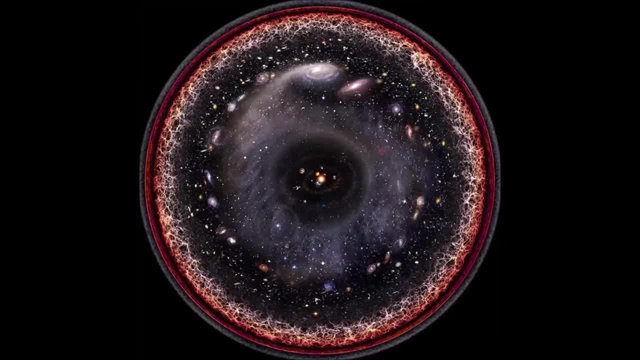 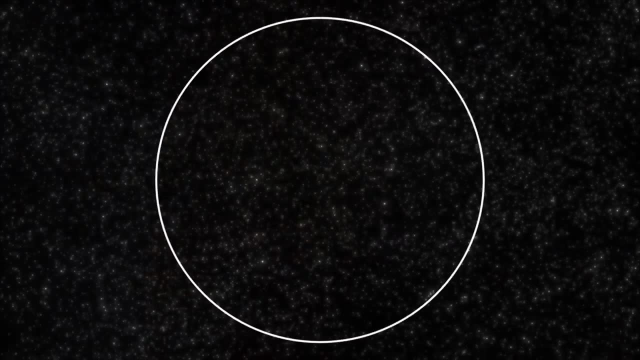 Because our Observable Universe is geocentric. the same is true of any planet in the universe. Every pointed space has its own arbitrary Observable Universe with radius of about 46 billion light years, marked by a cosmic horizon. This radius is determined not by how far away the most distant objects we have seen were when their light was emitted. 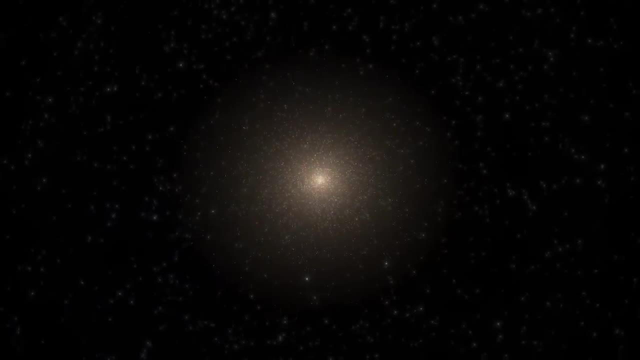 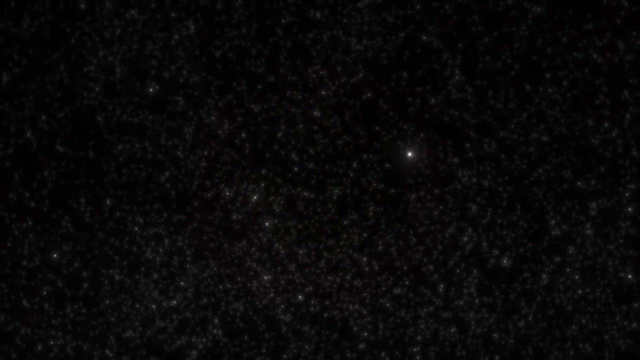 but rather how far those objects are estimated to be now, as the space between us and them has grown so much. since that light began travelling towards Earth, The most distant galaxies of the Hubble Ultra Deep Field have now receded to in excess of 40 billion light years away. 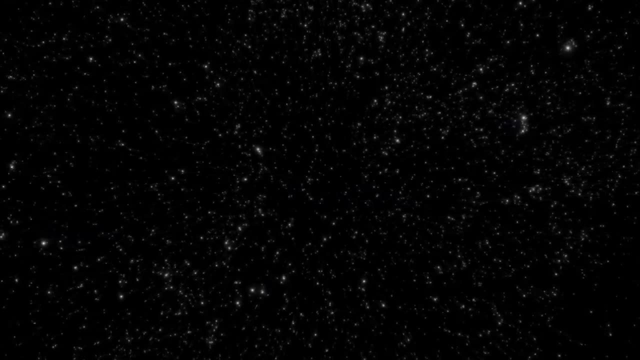 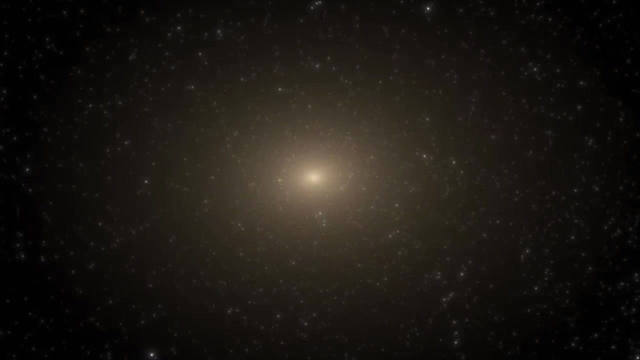 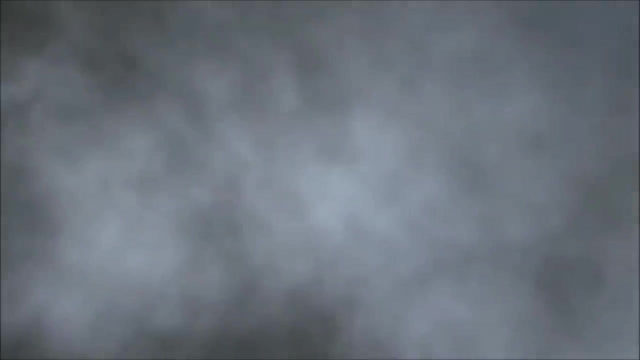 from Earth, and their light would never possibly have enough time to reach us. now, Beyond the cosmic horizon, light's speed and the universe's age are no longer compatible, and thus we are confined to our observable universe, segmented and detached from the full scale of the cosmos. 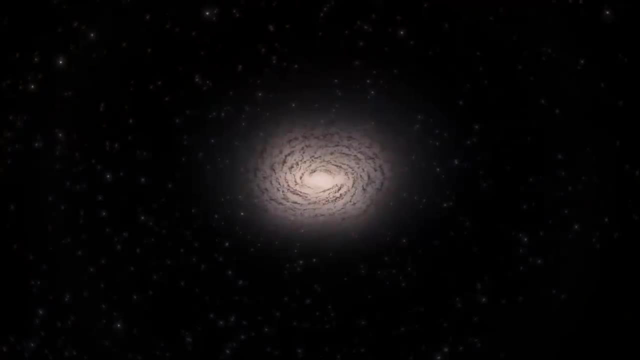 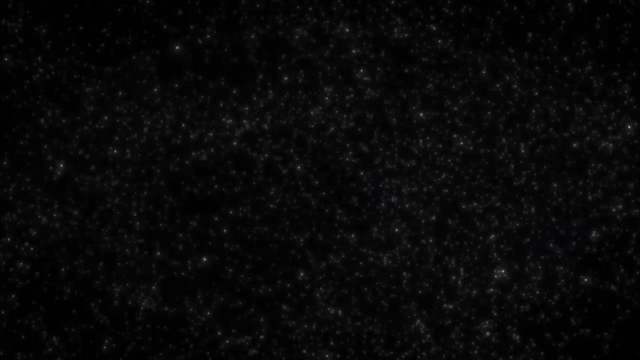 Because of this, we are unable to conclude on what could lie beyond the boundary, but given that the universe appears to be relatively isotropic on a large scale, you would expect more of the same- clusters and superclusters of galaxies. The real question: is how much of it is there? As you might expect, that's a very difficult question to answer, and the estimates we have so far depend on measurements of the universe's curvature and assumptions about its shape, which still represents a somewhat grey area in cosmology. 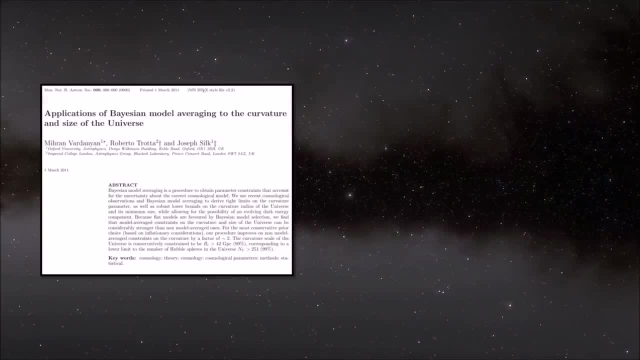 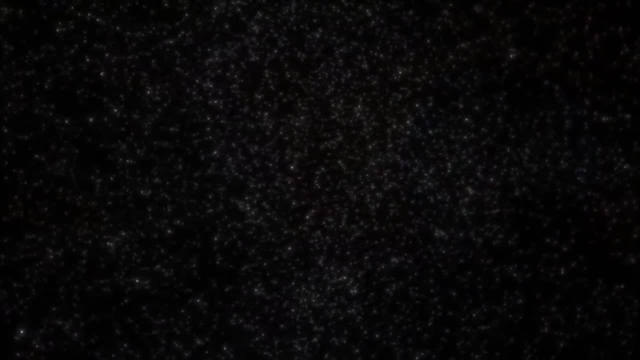 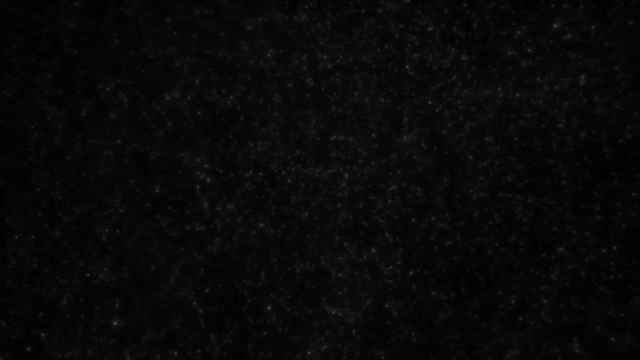 here. but, in short, the best estimate we have so far made by physicists at Oxford University is that the total area of the universe must be at least 250 times the radius of the observable universe. This puts the total diameter of the universe at over 23 trillion light years. 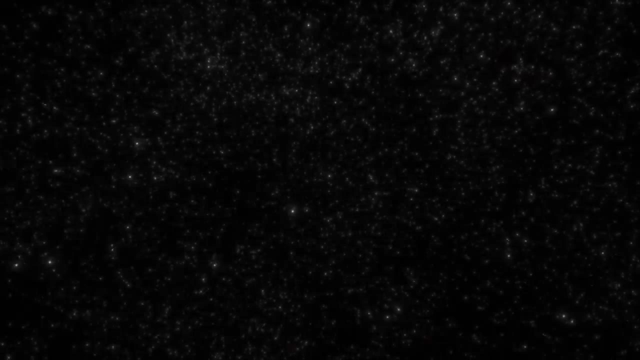 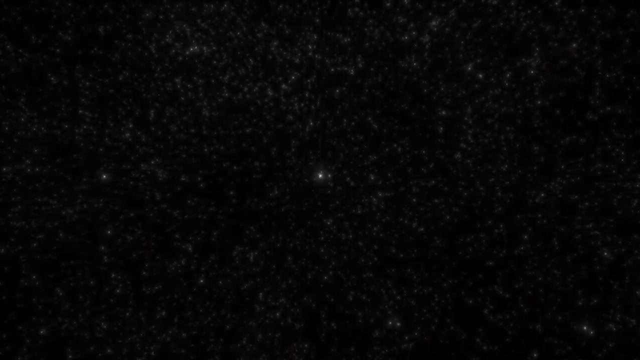 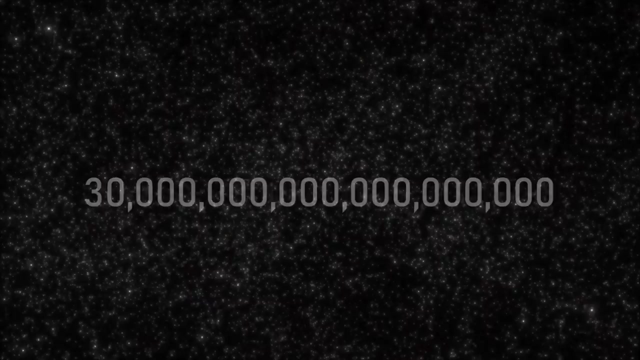 Which would mean that the 93 billion light year observable universe that we can see accounts for a mere 1, 15 millionth of its total expanse. If our observable universe is home to 2 trillion galaxies, then the unobservable universe may house as many as 30 quintillion of them In 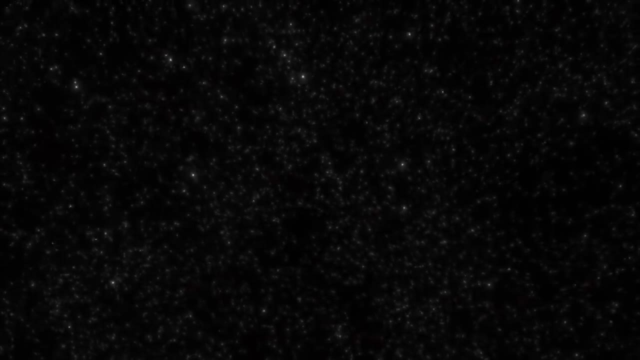 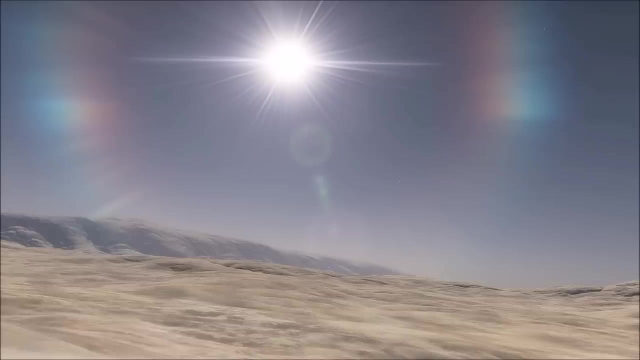 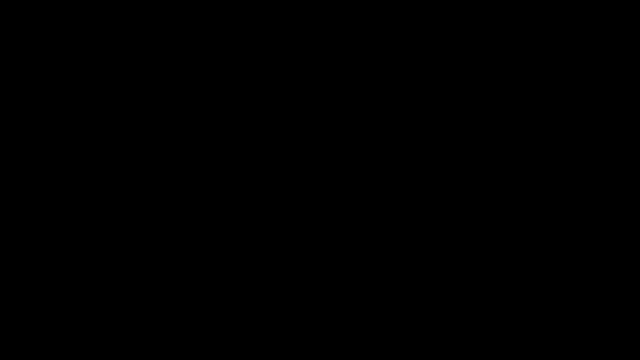 truth, we will probably never know the exact size of the total universe, but with the numbers considered here, it seems almost inevitable that somewhere else in space life must be playing out on another world. The discovery of the universe's expansion is one of the most important discoveries ever. 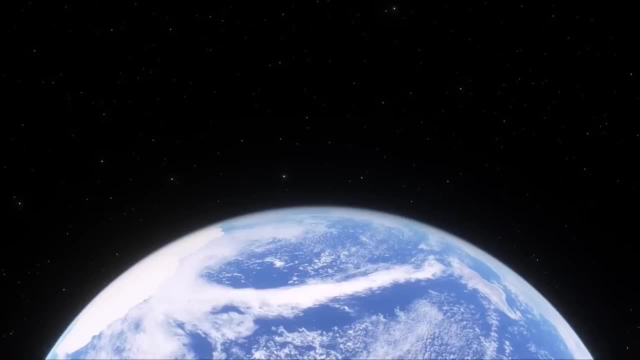 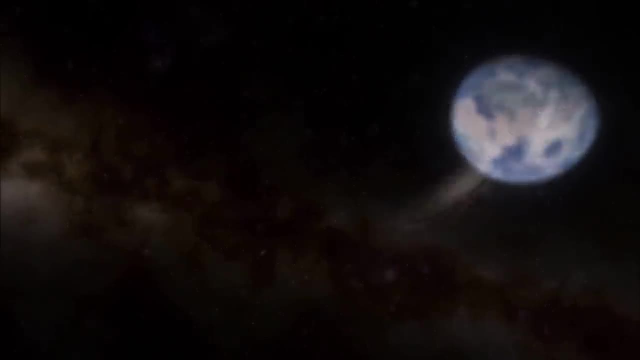 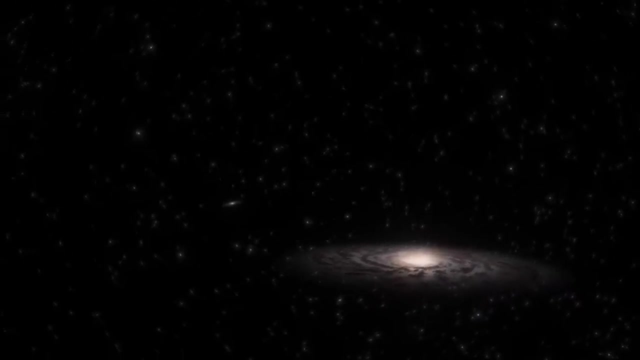 but we still didn't have the full picture For a long time. afterwards, astronomers expected that the rate of expansion would actually start slowing down as the galaxies on the inside begin to pull back against the universe's inflation. However, as scientists quested, 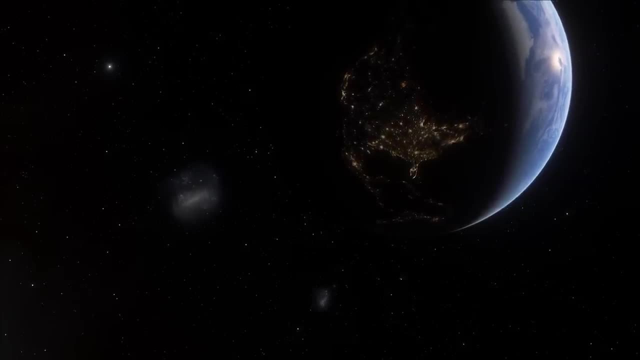 to establish a more accurate value for the whole universe. they were unable to do so as the galaxy's inside began to pull back against the universe's inflation. However, as scientists quested to establish a more accurate value for the Hubble constant, a startling discovery was made Since Hubble redshift surveying. 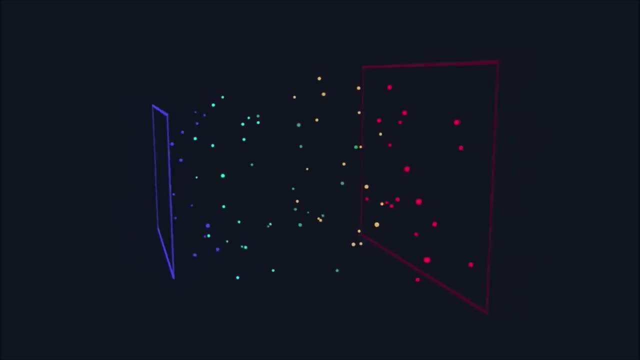 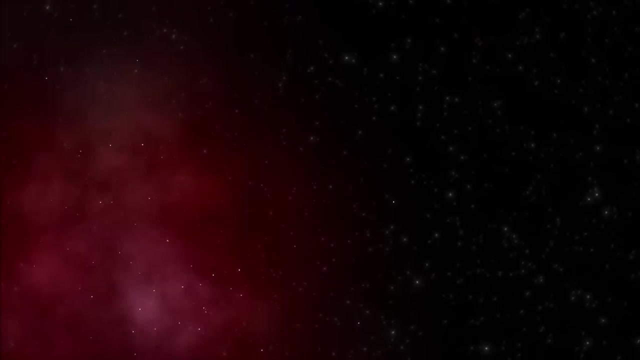 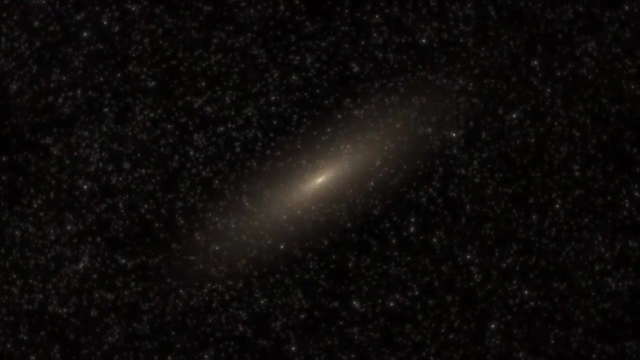 techniques have improved significantly and we can now detect galaxies not just millions of light years away, but billions, Because redshift is indicative of the universe's expansion. we can compare a galaxy's distance with its redshift to determine how much the universe has expanded at the different stages of its evolution. But that's easy enough. 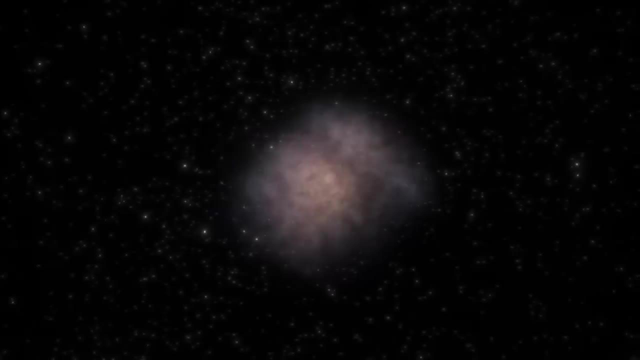 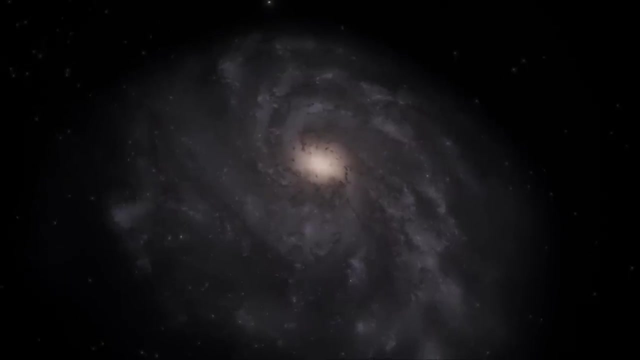 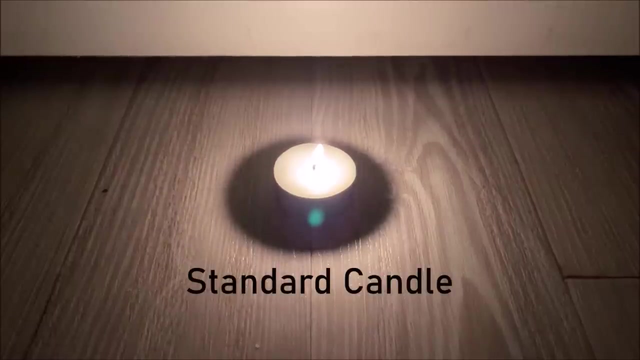 but that's easier said than done, because galaxies vary in brightness so much so it becomes very difficult to estimate their distance precisely. A more suitable means to measure cosmic distances would be to take something with a known absolute magnitude, known as a standard candle, and calculate its distance by analysing the dimness of the object relative. 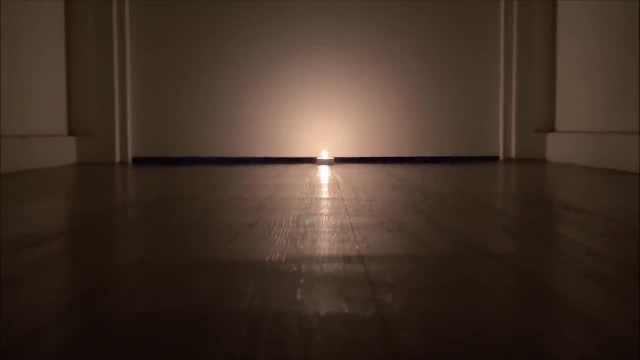 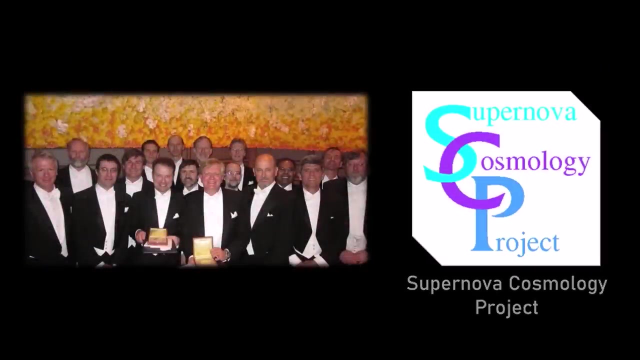 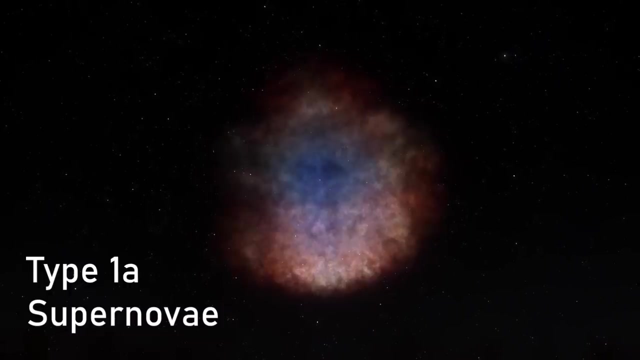 to how luminous it should be. With this in mind, two separate projects, the Hi-Z Supernovae Supernova Search Team and the Supernova Cosmology Project- both attempted to measure the expansion of the universe over time by using distant Type Ia supernovae as standard candles Type. 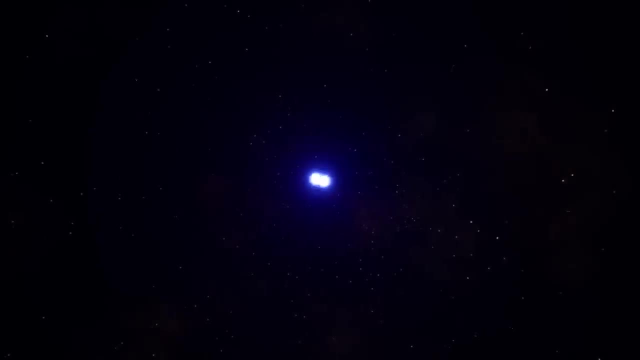 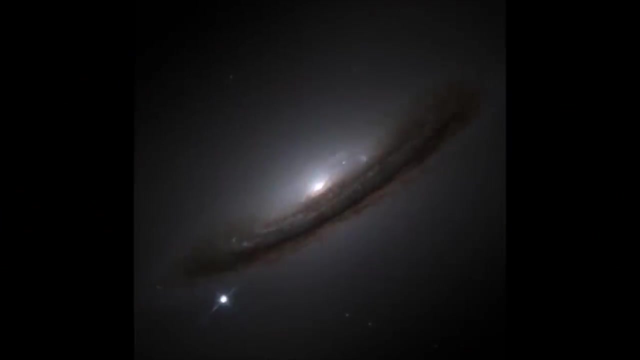 Ia supernovae are superluminous explosions caused by white dwarf stars in binary systems. They have a relatively consistent brightness and can outshine their entire galaxy. Using these stellar ghosts as calling cards, the two projects have been able to measure the 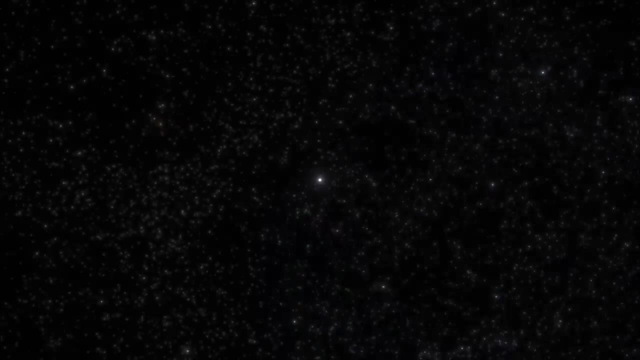 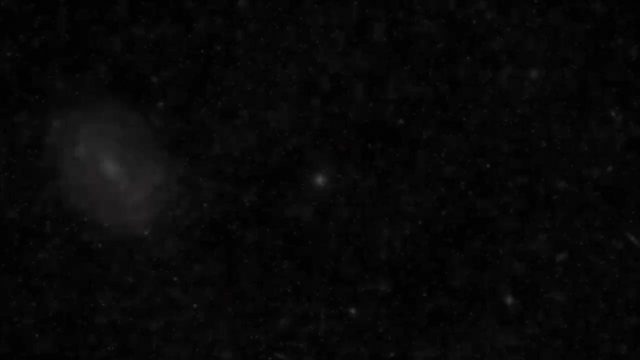 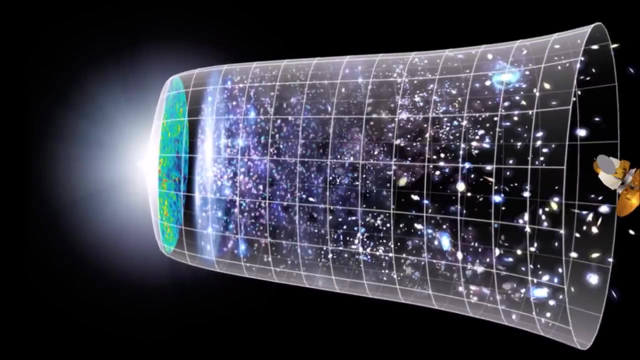 distances of far out objects and then compared this with each objects respective redshift values. The unlikely result was that the very distant objects seemed to be much further away than the more local objects. It's as if the universe has expanded more in the latter. 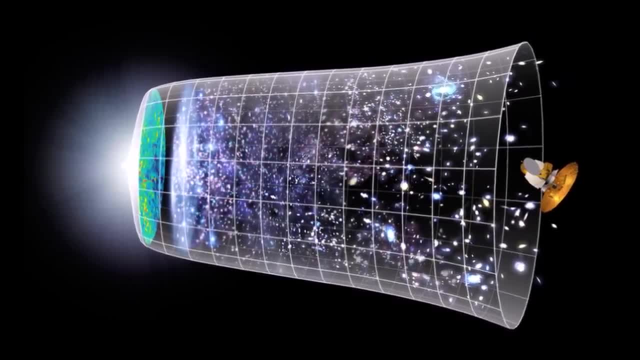 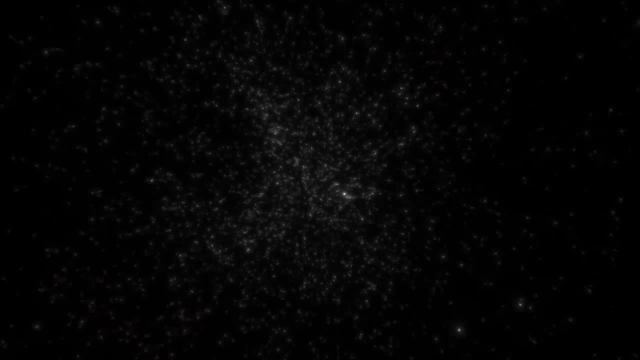 half of its life, Or rather, its expansion is accelerating. We know that our universe has been expanding at different rates based on what it has been through in its life, and at one point it did look to be slowing down, as it was once predicted to do so. 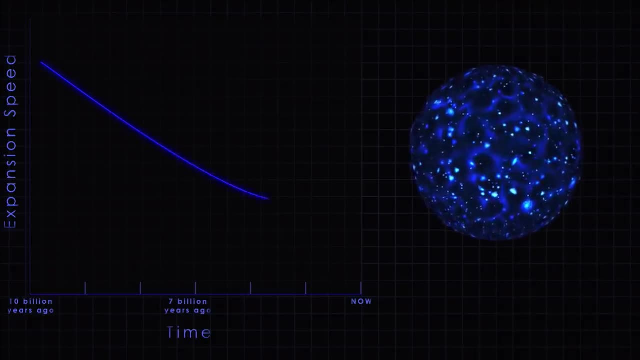 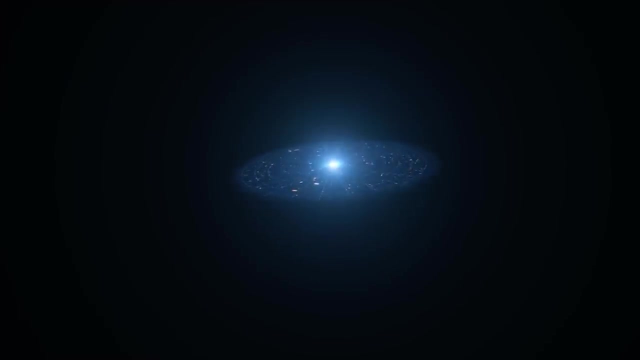 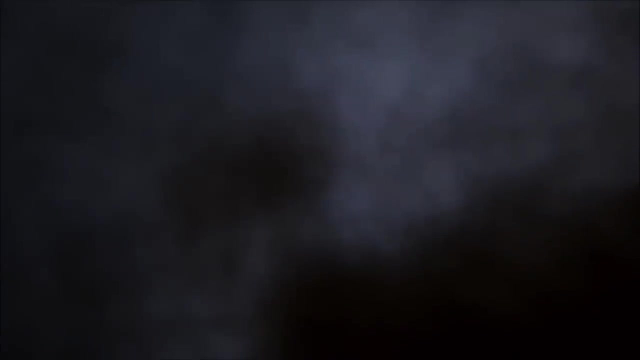 But then, around 4 billion years ago, and for a completely unknown reason, an invisible force began to hijack the universe's growth, causing its expansion to accelerate, leading to more aggressive expansion in its recent few billion years. Moving into the 21st century, we had opened. 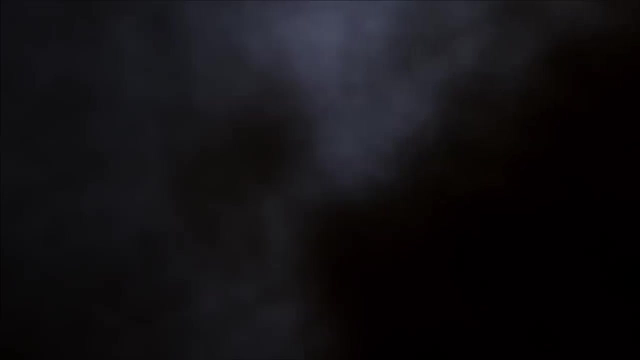 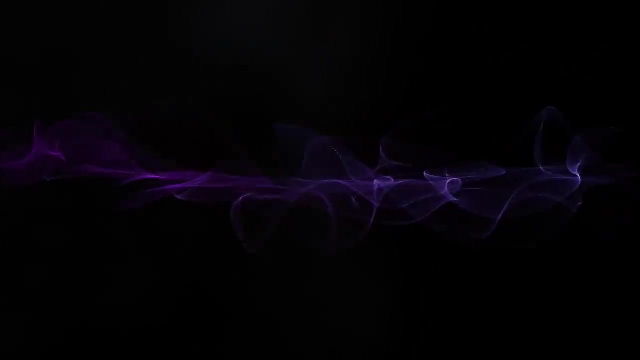 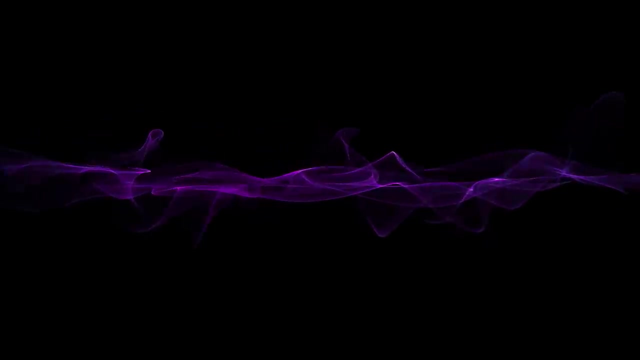 the path to a new paradigm of astrophysics- the study of dark energy. Dark energy is the term given to the invisible force that is responsible for the accelerating expansion of the universe. We know barely anything about it, save for that it appears to work like an anti-gravity force. 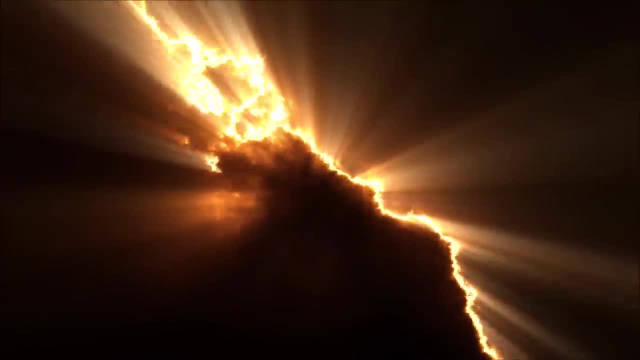 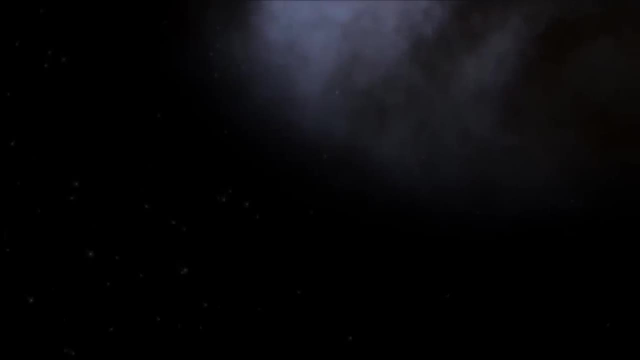 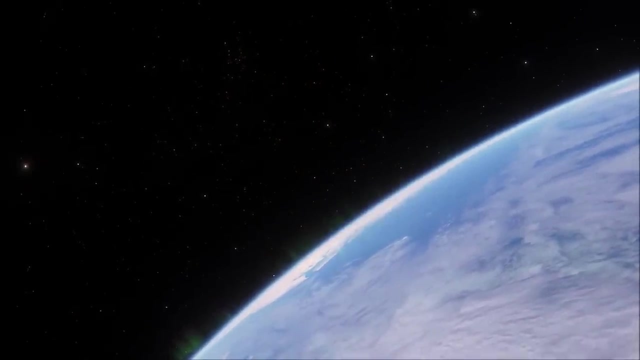 It exerts a negative repulsive pressure that behaves inversely to gravity, which is aiding the universe's expansion rather than slowing it down. Dark energy is notoriously hard to study- it does not interact with light, so it cannot be seen nor detected, and there are many hypotheses describing its nature. 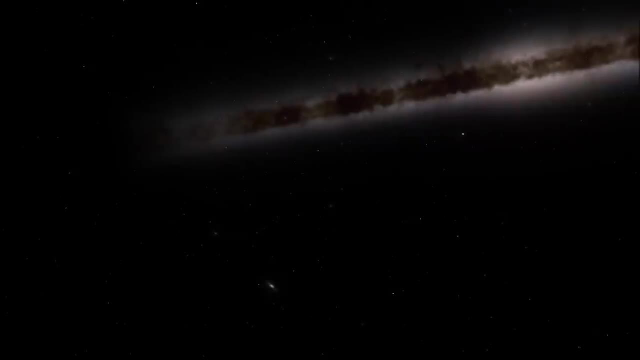 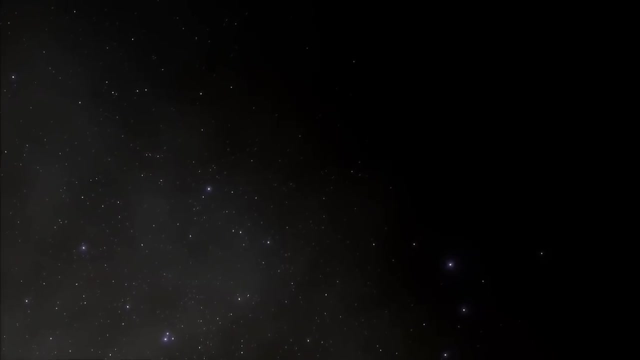 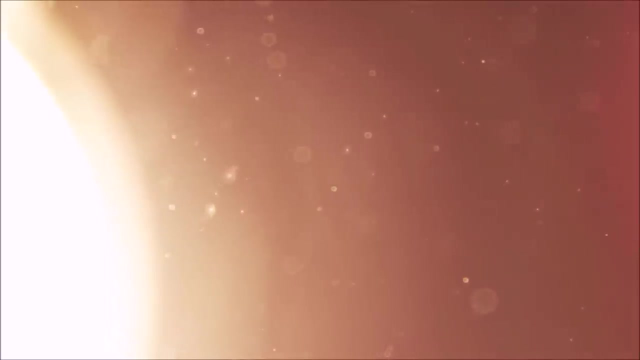 and prevalence. But what we do know is that around 9.8 billion years of cosmic time, this energy became the prevailing energy in the universe, marking the beginning of the dark energy dominated era In the early universe. radiation dominated its behaviour Then for almost 10 billion years. 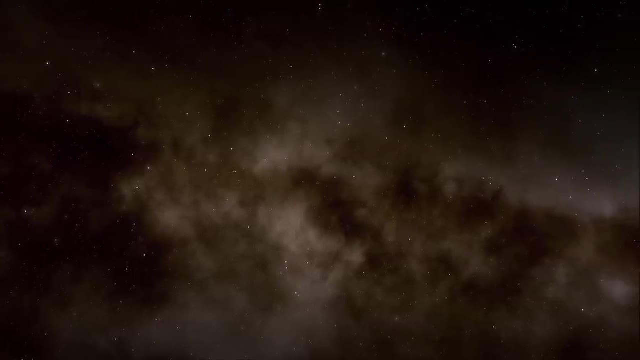 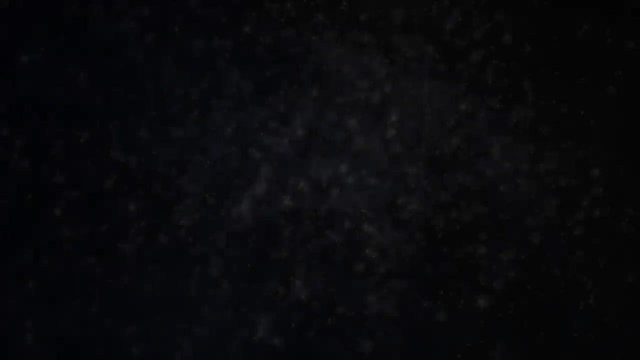 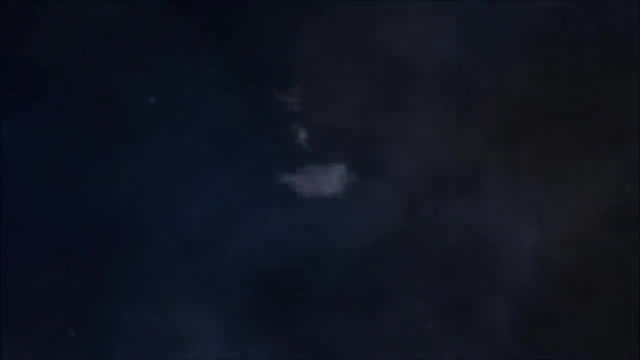 matter was the dominating influence. However, as the universe has expanded, the density of matter has been falling as it has been spread more sparsely. Dark energy, on the other hand, is believed to remain consistent in its density, meaning more of it pops into existence proportionally as the universe expands. 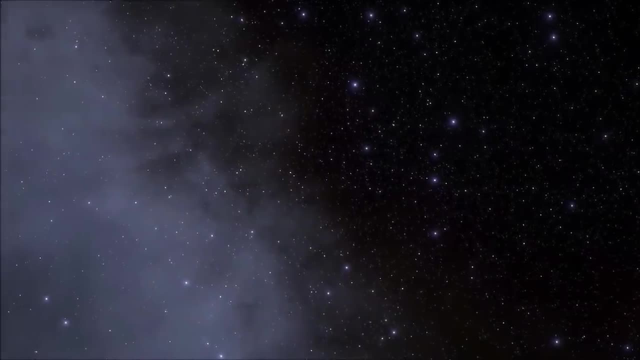 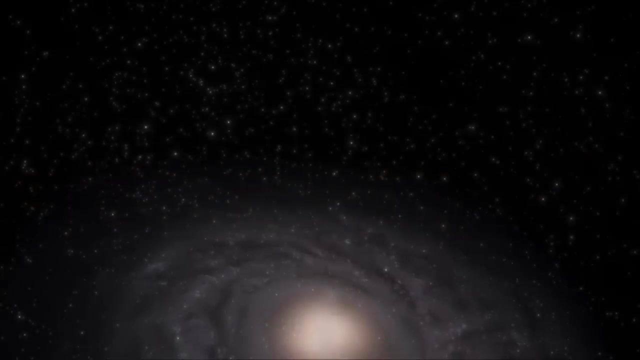 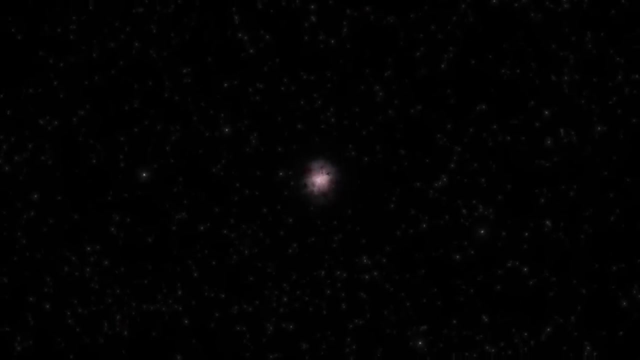 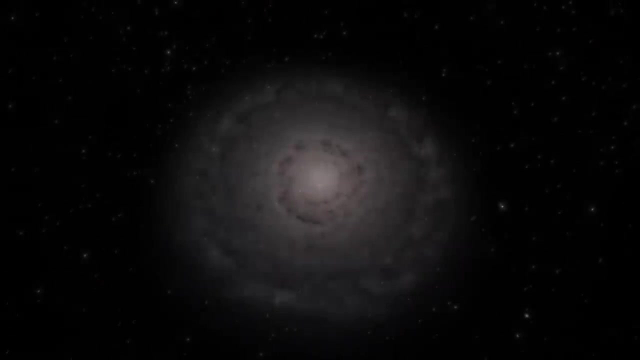 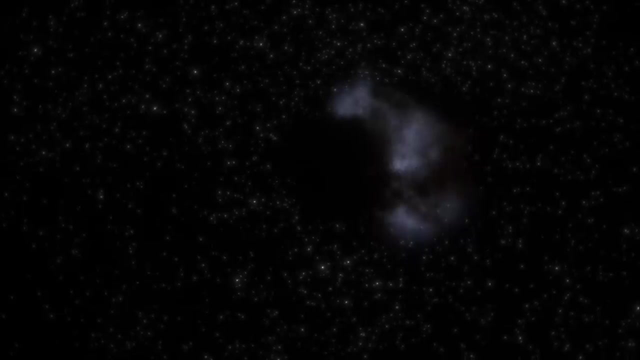 Thus there came a tipping point around the universe's expansion. On a local scale, the expansion of the universe is very weak, and so gravity is able to keep objects such as galaxies held together regardless of how big the universe becomes. However, the massive cosmic voids between galaxies and galaxy clusters are growing. 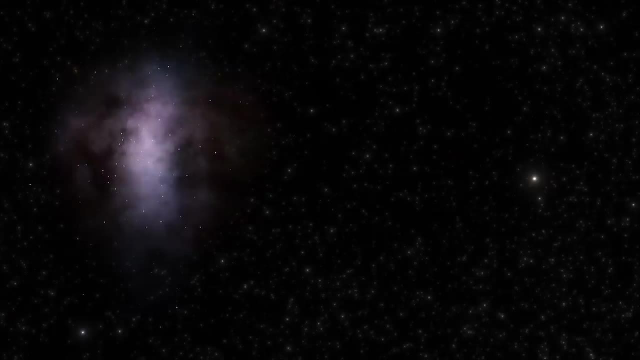 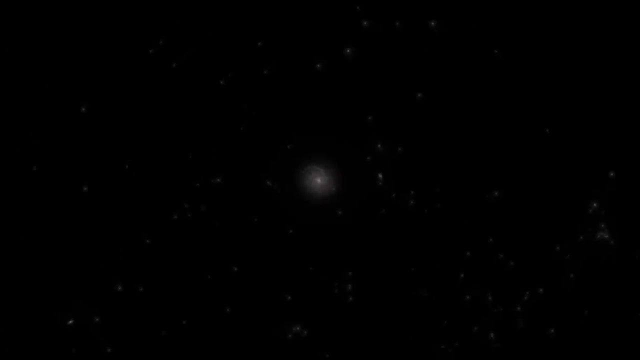 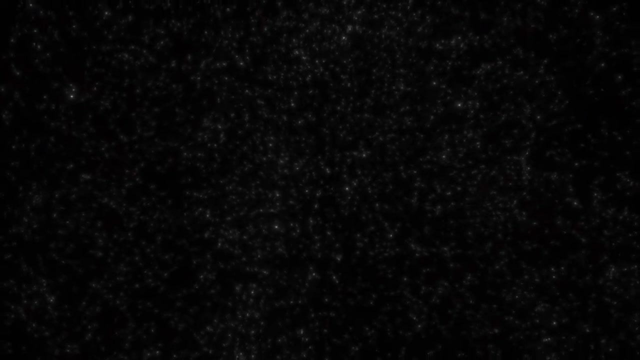 from within their dark interiors, gradually separating galaxies and galactic groups like our local group into their own isolated pockets of space. But because the expansion of the universe is accelerating thanks to dark energy, in time space will be growing so quickly that even our nearest galaxies will recede away from us much. 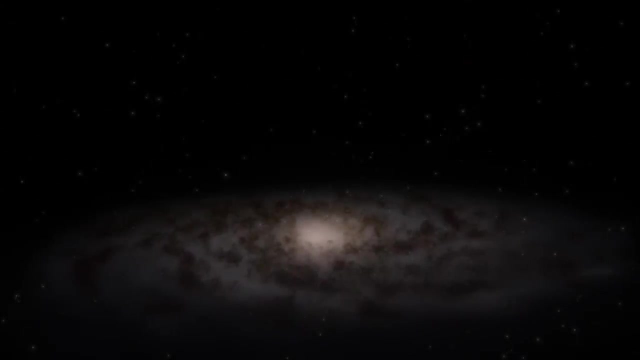 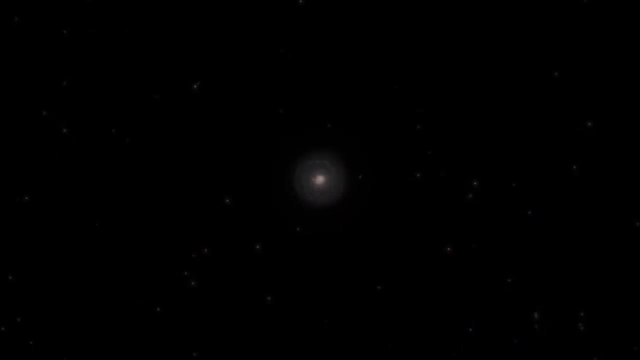 too quickly for their light to be able to reach us. This is the reason why the universe is so far away from us, and the cosmic horizon will begin to draw inwards Gradually. galaxies at the edge of the observable universe will start disappearing from view, as their light is no longer. 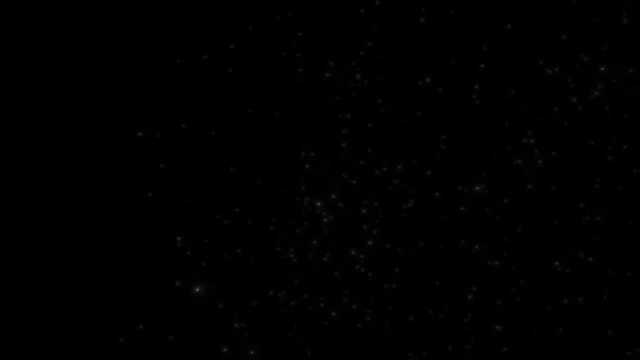 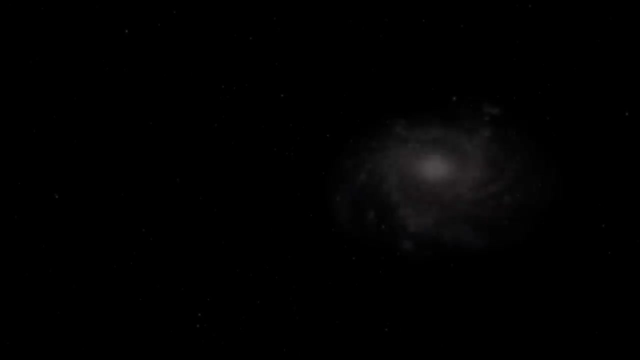 able to keep reaching the solar system, and the cosmic horizon will begin to draw inwards. This will continue until even our nearest galaxies are flung beyond the cosmic horizon, rendering even our local universe invisible In the very distant future. every galaxy's view of the universe will start and end with its own stars. 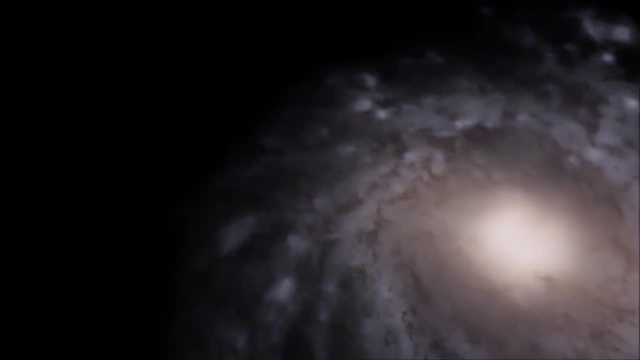 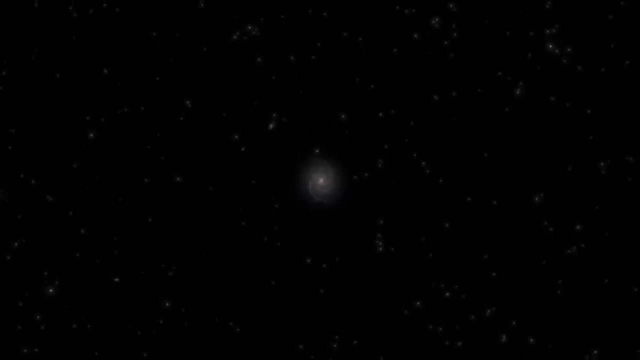 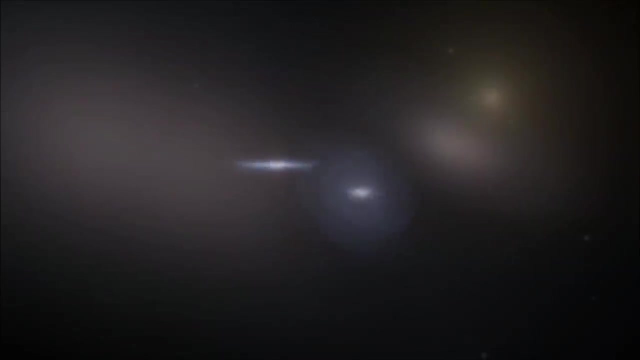 with nothing but empty darkness beyond the outer rims. We will never see another galaxy again. With galaxies separated from one another, they will not be able to merge and will thus eventually stop producing new stars. The Milky Way and Andromeda galaxies will merge before any of this happens, but after that. 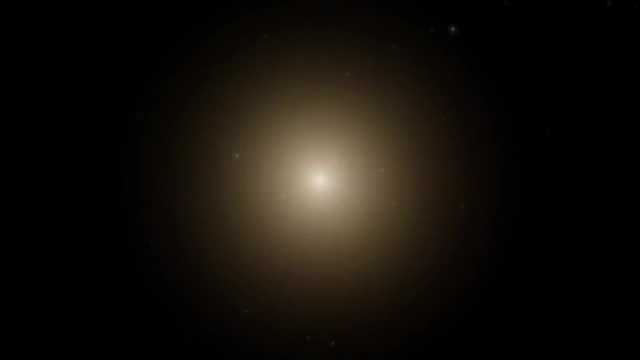 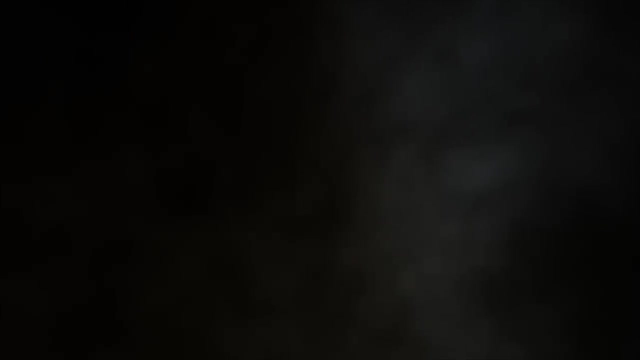 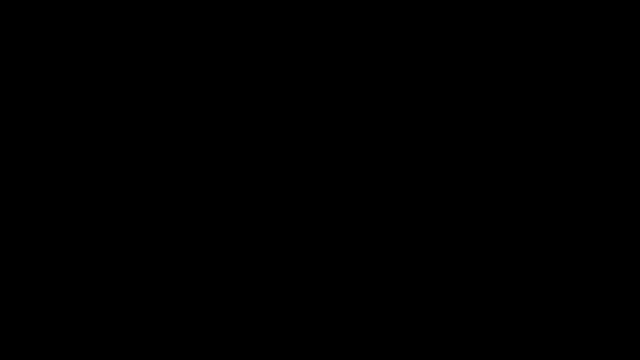 the resulting elliptical galaxy will gradually burn through the last of its stars. Inevitably, the day will come when the last stars of the universe have either gone out or exploded, bringing the universe into a second eternal dark age. Ultimately, the universe's energy will be lost through natural processes. 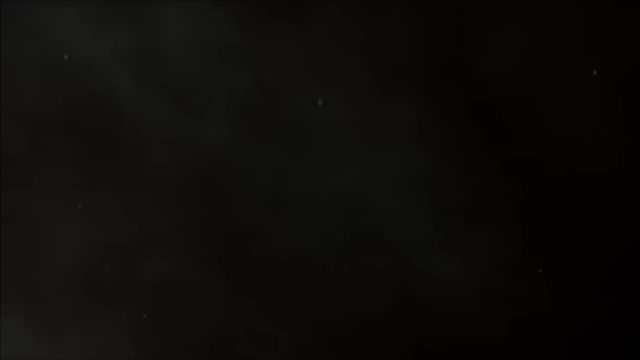 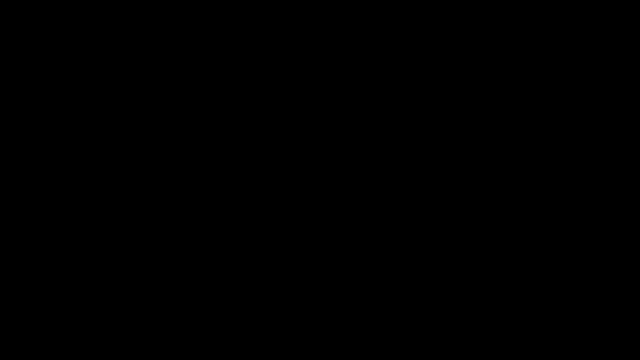 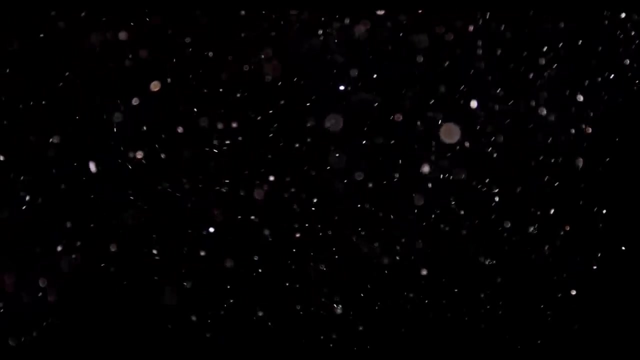 until nothing is ever able to happen again, The universe will reach its heat death, the ceasing of all heat and energy exchanges. Thereafter, the universe will be a totally homogenous, incomprehensibly large and boundless void, eternally dominated by dark energy. 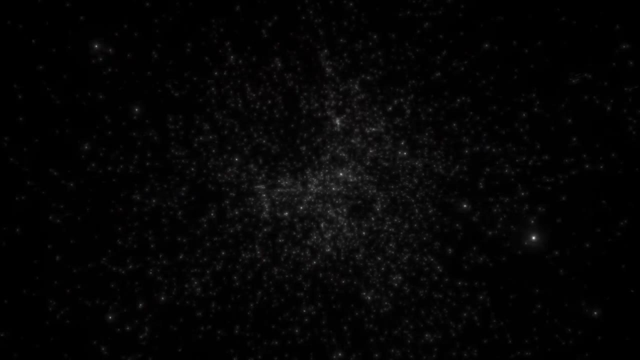 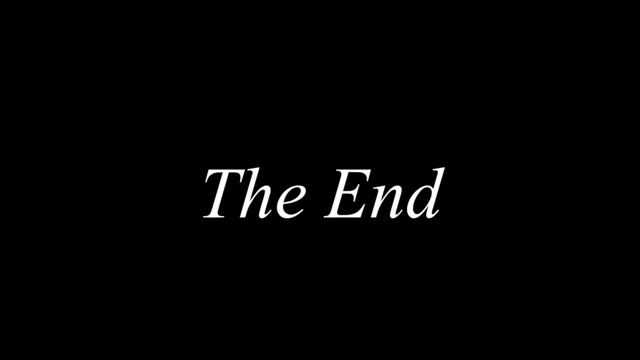 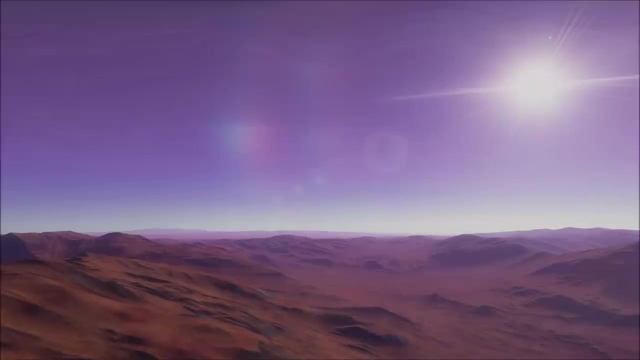 A bit of a depressing ending, to be sure, but there you have it: the fate of the universe in the Age of Darkness. Thank you for watching and I'll see you in the next video.